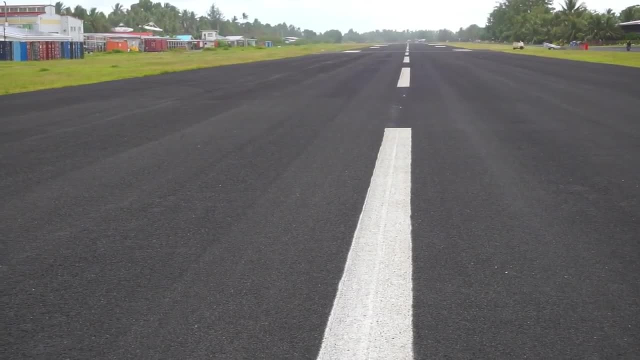 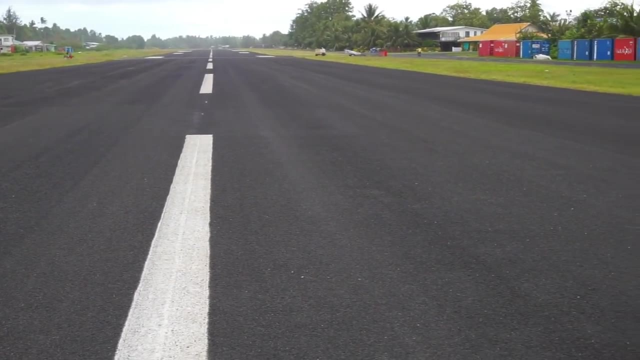 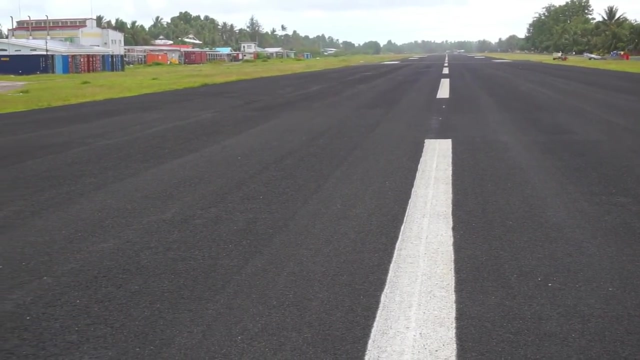 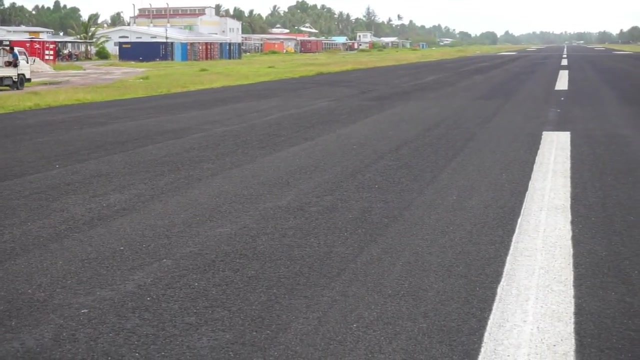 And here's the runway of the International Airport here in Funafuti, the capital of Tuvalu. There are only two flights that come in to this airport a week, both from Suva in Fiji- One flight on Tuesday and one flight on Thursday- And this runway that you see here is the. 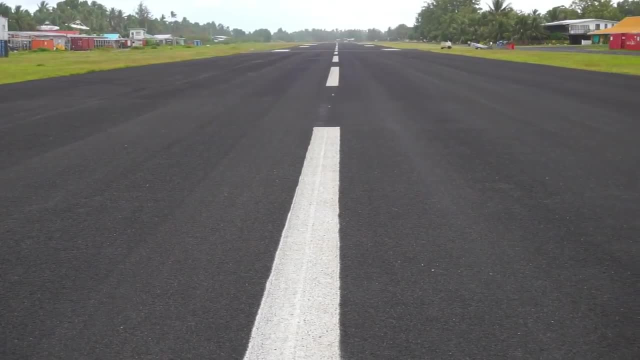 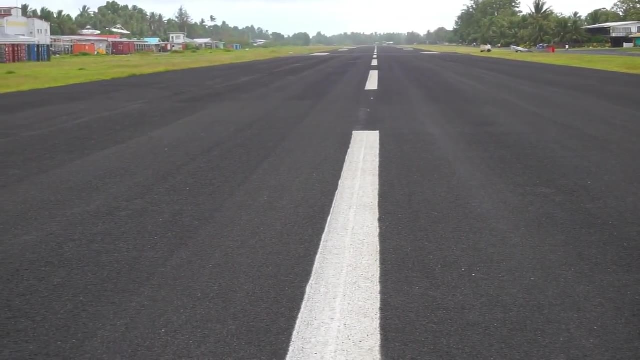 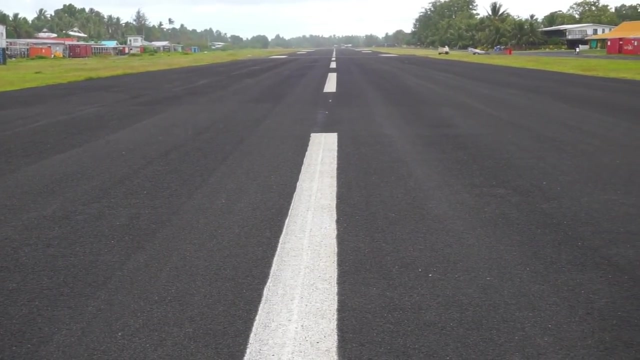 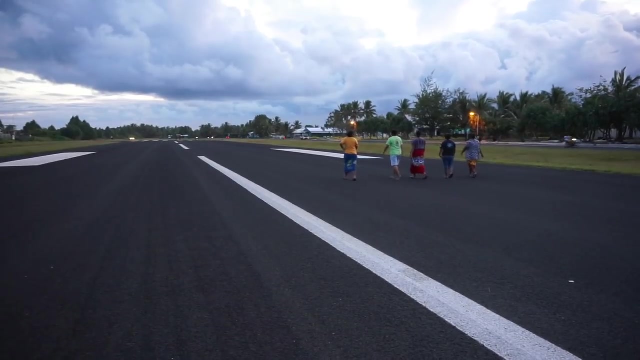 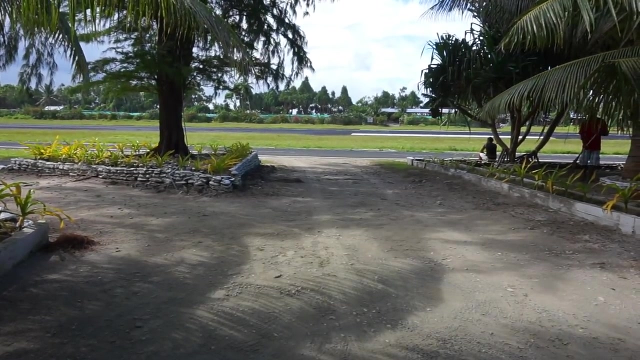 center of social activity in the evenings right about sunset time, And there is a video dedicated to what's happening here on the runway every day around sunset. But here it is now early in the morning And right there in the middle near the frame. 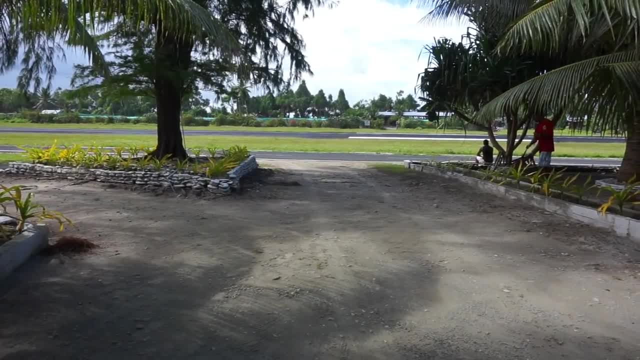 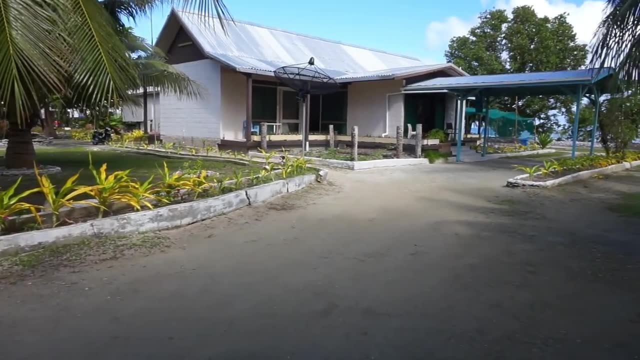 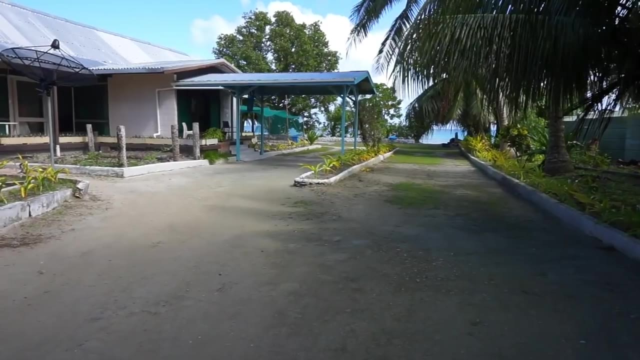 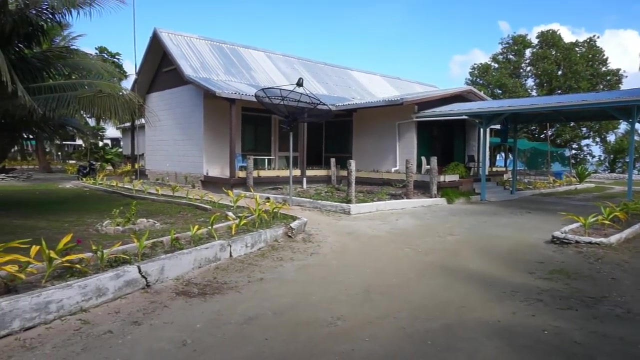 you can see the runway on the international airport and here is the Prime Minister's House, right there, and that's the lagoon of Tuvalu, The sea that you see there, and here is the house once again: Volcanoes 모두 круп knit. 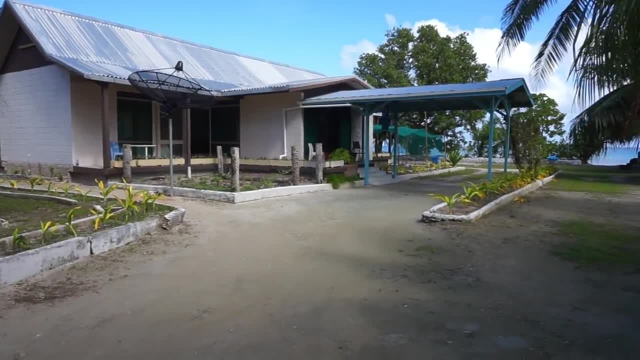 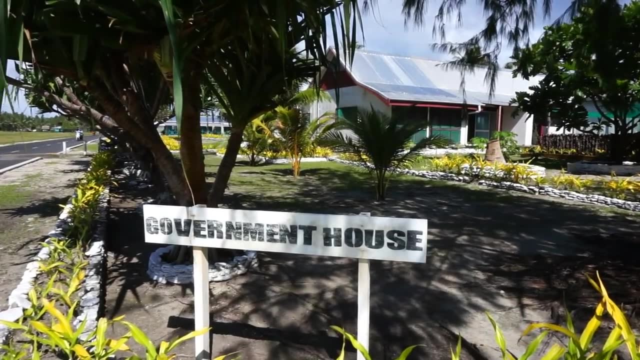 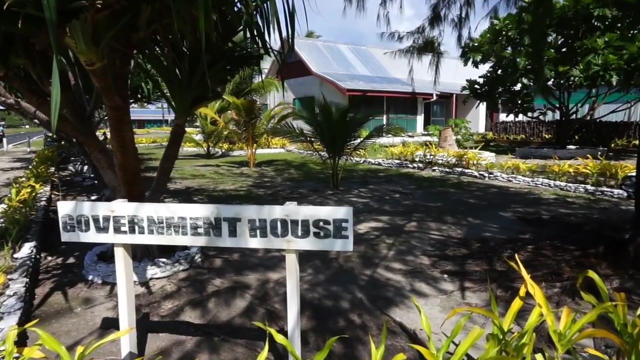 Verurs assimile was nghĩa like otra para tenemos Little Visual, American and signed by Mysterio. similar to the White House in Washington, right next to the Prime Minister's house, you will find the government house that you see here, right there, and this is the. 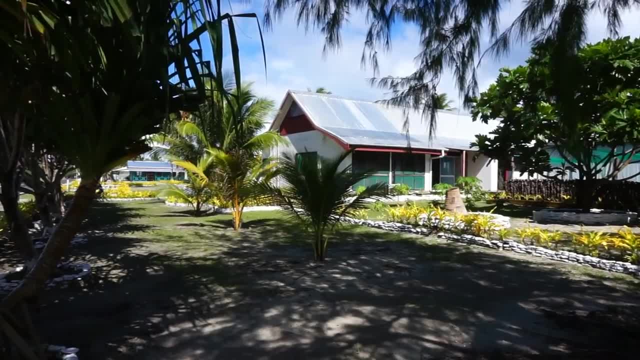 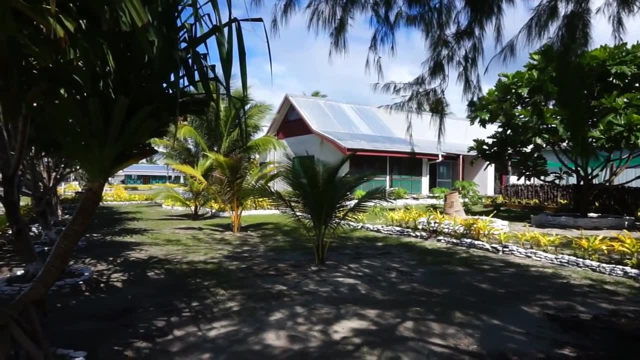 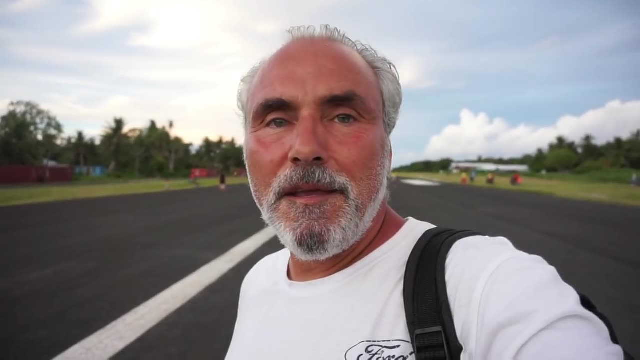 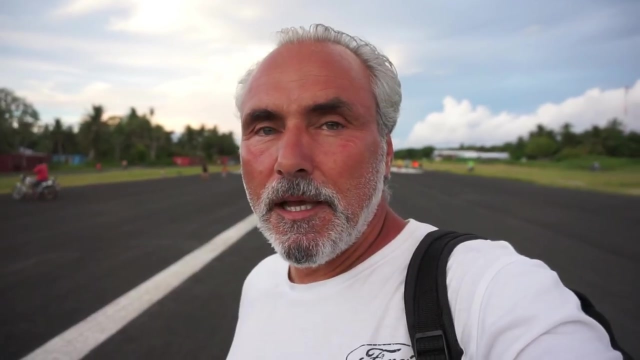 residence of the governor of Tuvalu. the governor, of course, is the representative of Queen Elizabeth, the second here in Tuvalu. and here are a couple of interesting facts about Tuvalu. the whole country has about 12,000 residents or citizens, and the population has doubled since 2002. 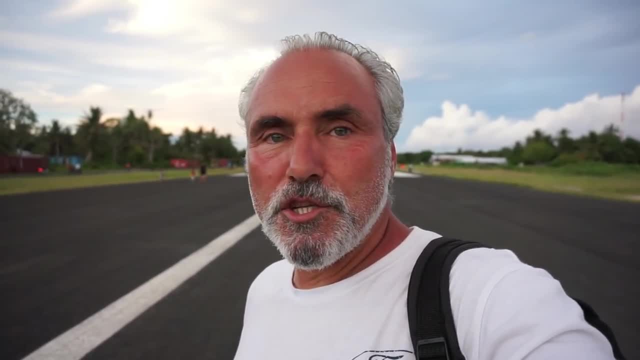 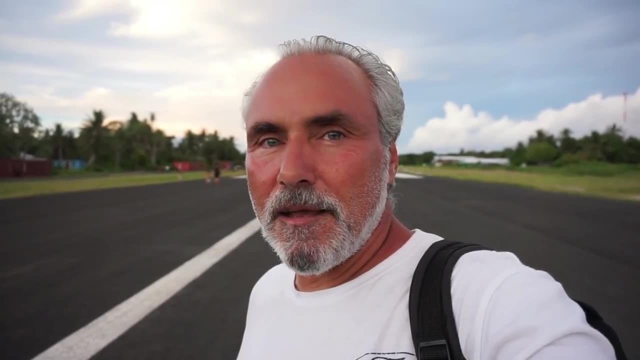 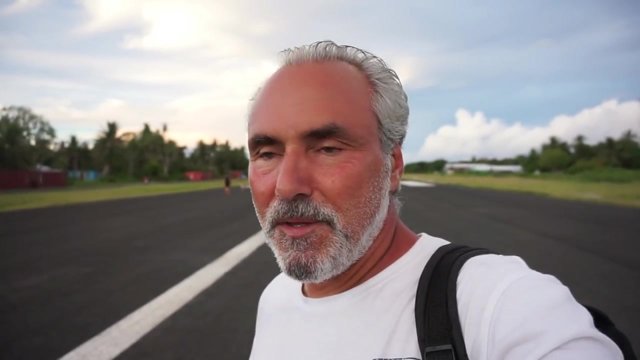 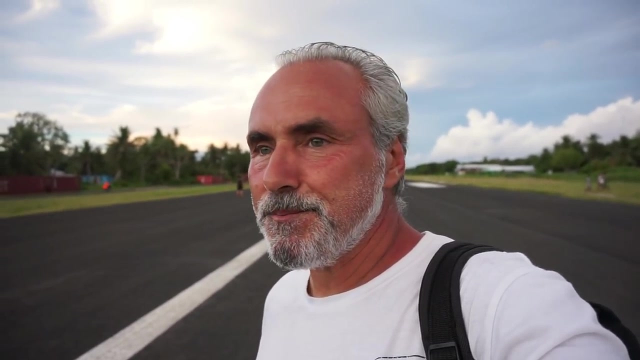 the country consists of nine islands, of which six of them are atolls, meaning sandy or coral based islands, and the other three are coral reefs, and the whole country has about 10 kilometers of paved roads. they're also a mix of Polynesian and Melanesian- the residents of Tuvalu that is, and here's a beautiful view of. 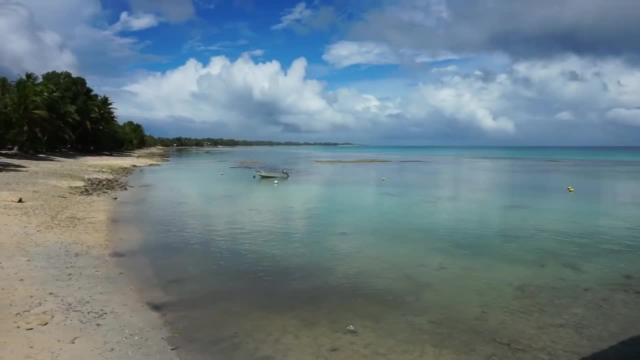 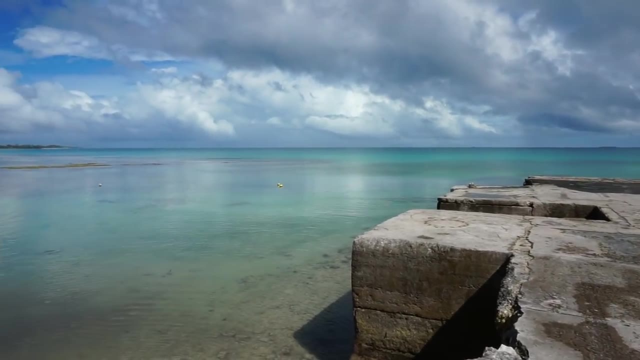 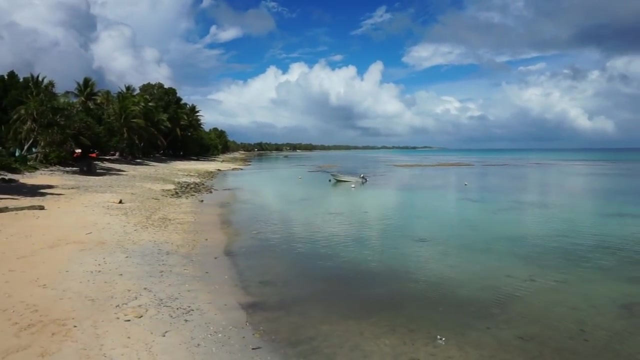 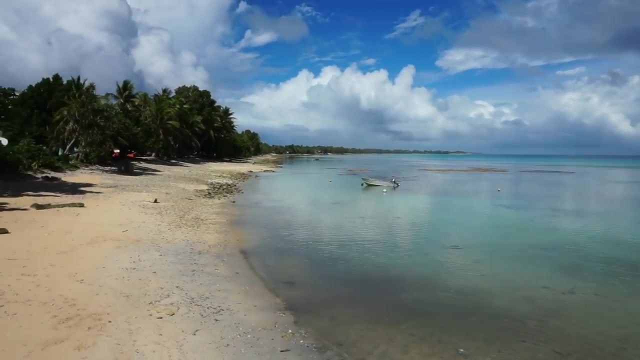 the Funafuti Lagoon. here's the main wharf, right behind the government building here in Funafuti. I'm not far from the runway of the International Airport, which is a couple hundred meters behind me, and this is the southeastern direction. right there now the older people here in Funafuti in. 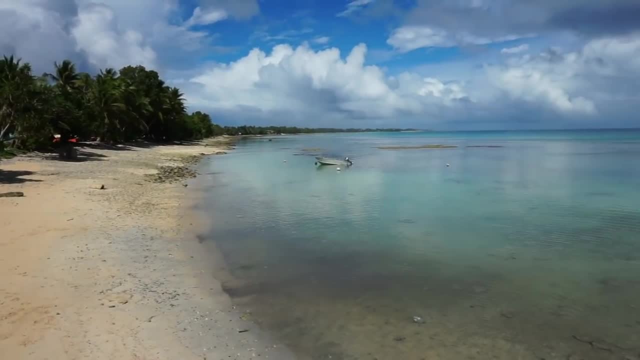 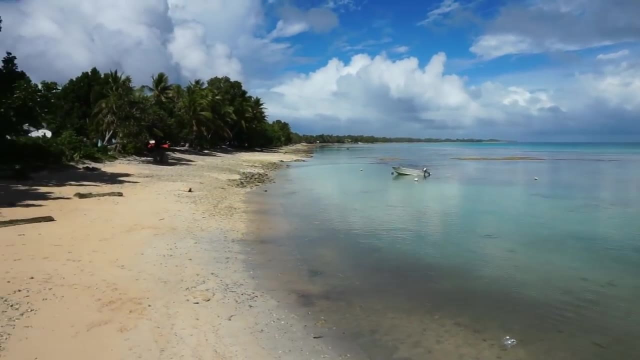 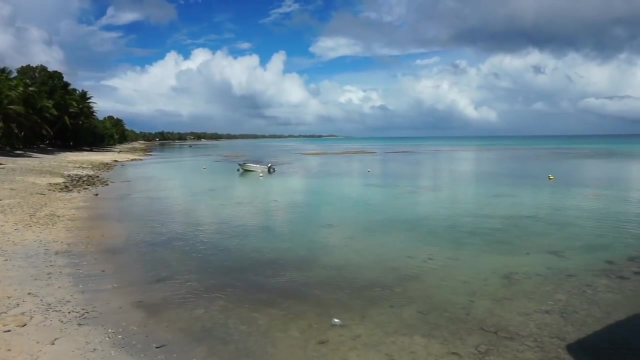 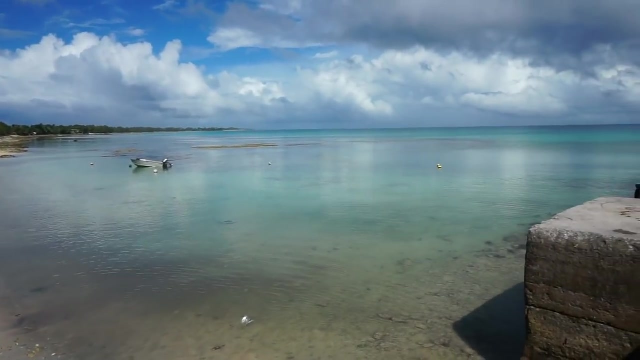 Tuvalu will tell you that 20 years ago they were able to come here and play football games on the beach, and this is low tide and you can see that it's almost impossible, even a low tide, for them to play football games here. now the beach has been lost at. 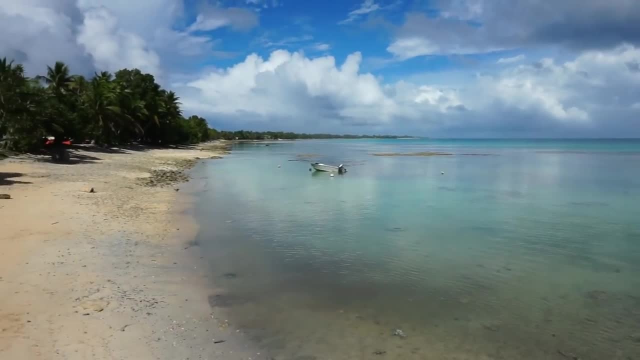 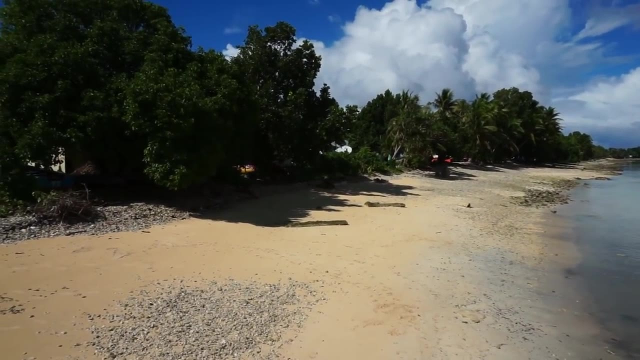 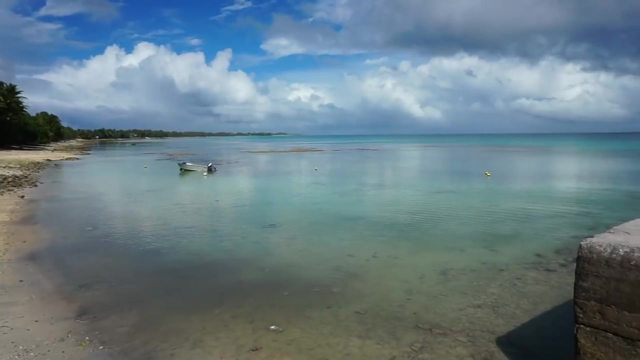 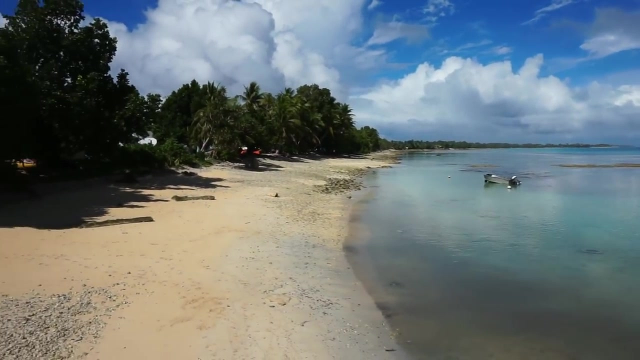 least about a hundred meters, and the rising sea levels are threatening to overtake the beach, the mainland of Funafuti, right here. so there are three countries here in the Pacific that are facing imminent danger from rising sea levels: the Marshall Islands, the Republic of Kiribati, Kiribati and Tuvalu. in about 20 years. 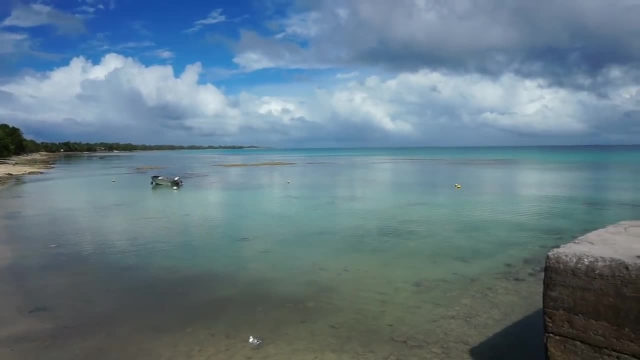 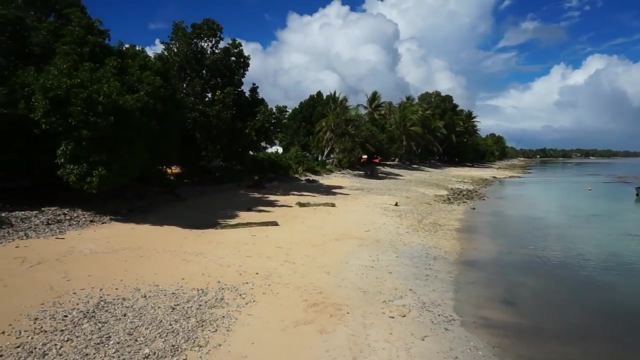 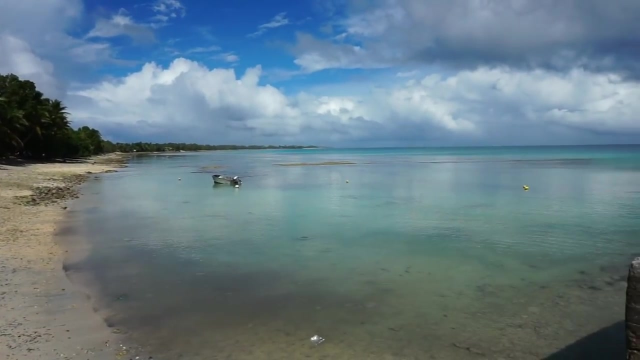 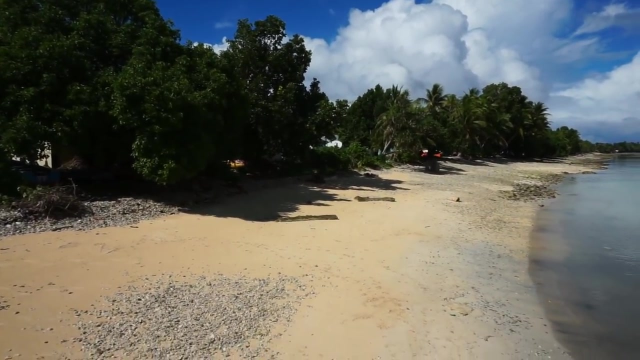 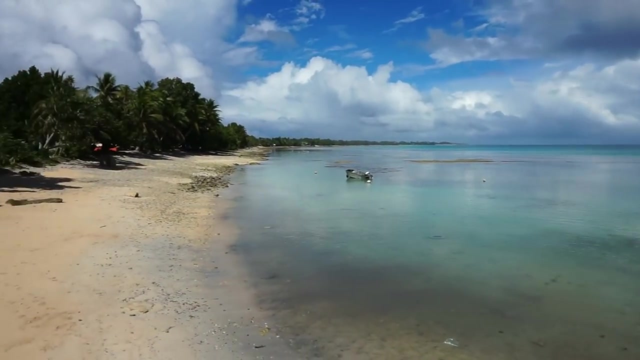 it is very doubtful if they can keep their country from sinking or being covered by seawater, and that's a very sad fact that you have to face when travel, when you travel to these three countries I just mentioned, at high tide the water comes very close to the houses over there, about five meters. 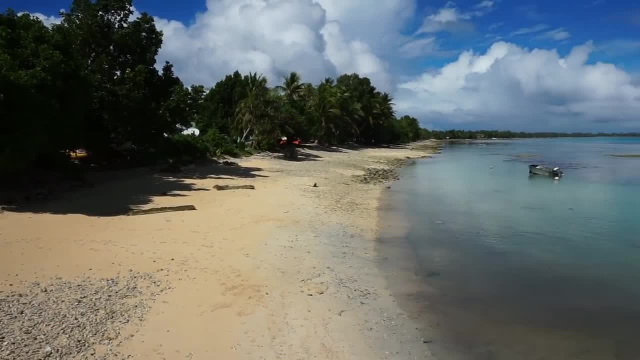 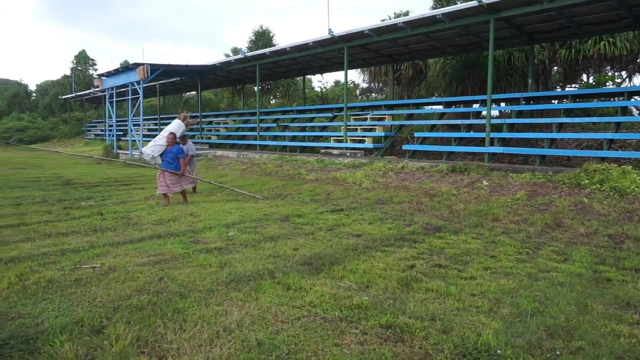 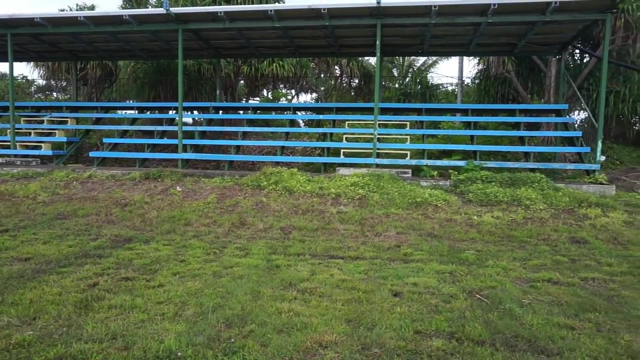 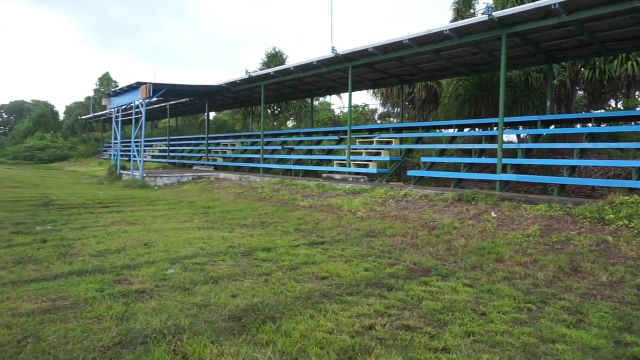 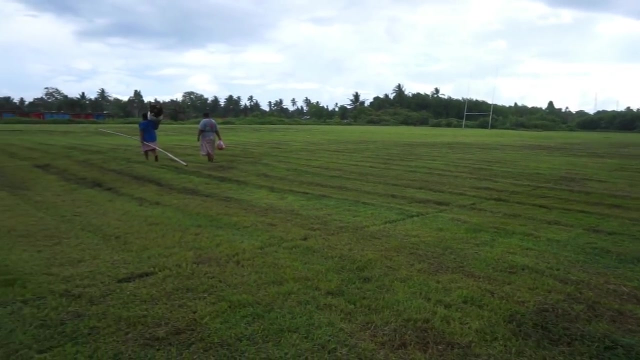 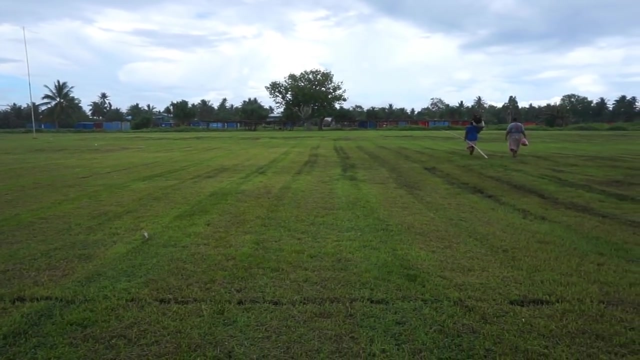 away and this beach gets covered almost completely. and here you see the stadium here in Tuvalu, in Funafuri. this is the national stadium, these are the seats and these are the grounds here for rugby. and in about 200 yards, directly ahead of me, is the runway of the International. 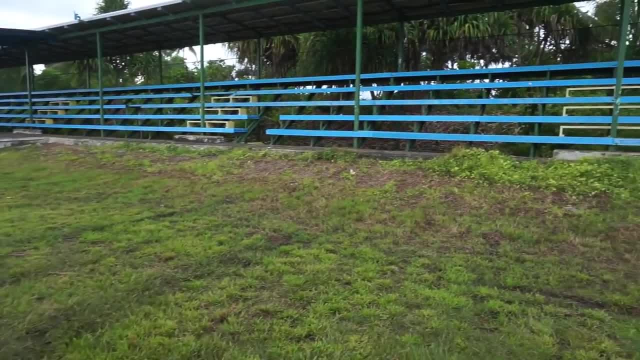 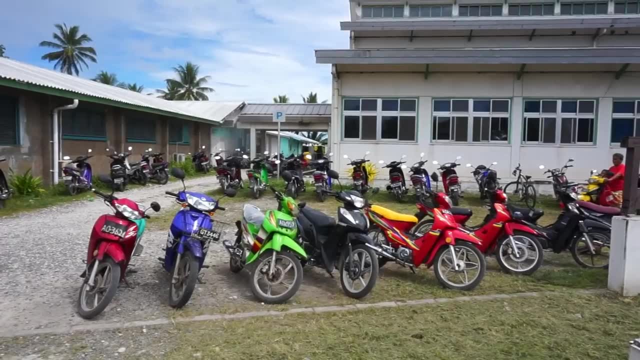 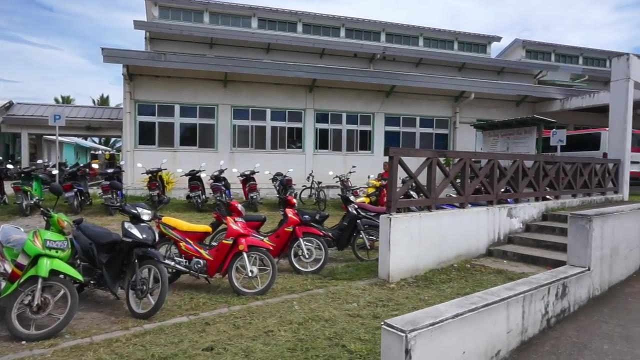 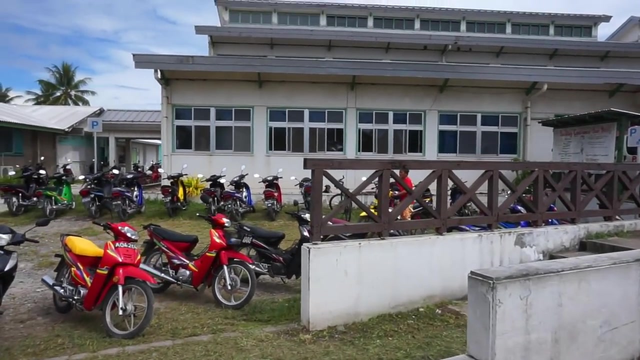 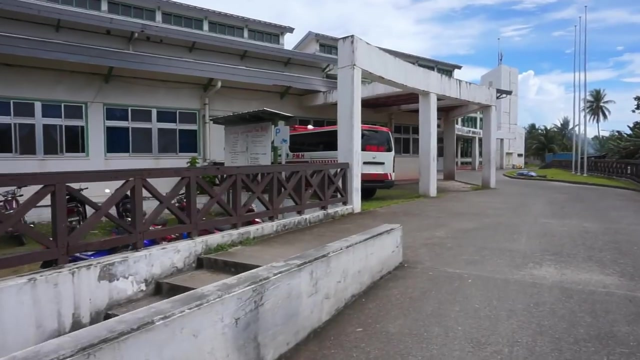 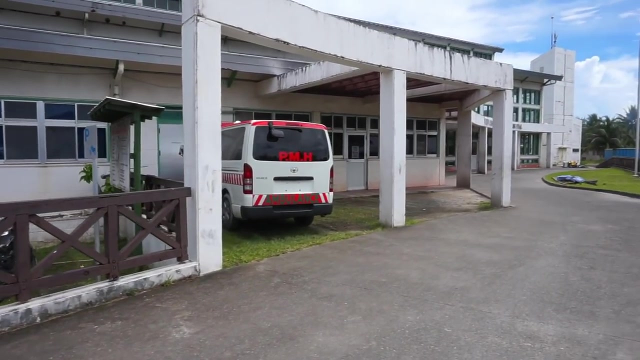 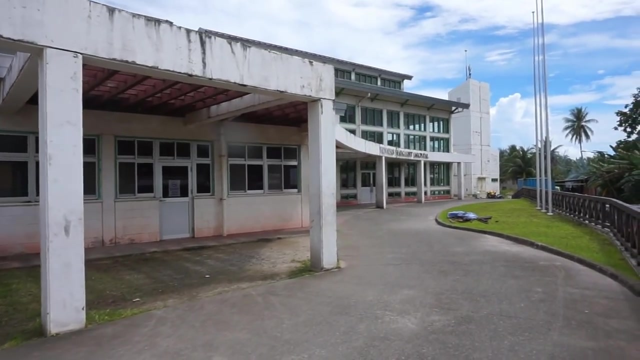 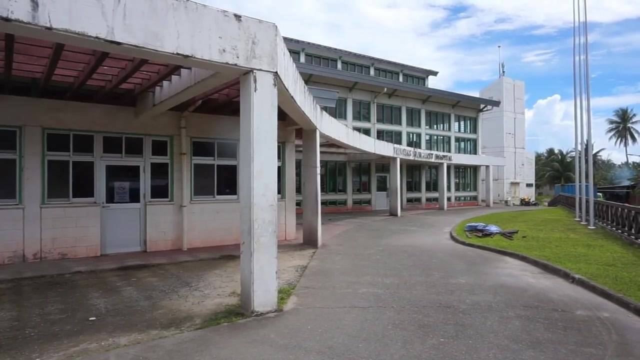 Airport and here's the hospital of Funafuri, the biggest hospital in Tuvalu. you can see all the motorbikes parked here and here's the ambulance of the hospital. here here's the general view of the building and the sign above the entrance says Princess Margaret Hospital. 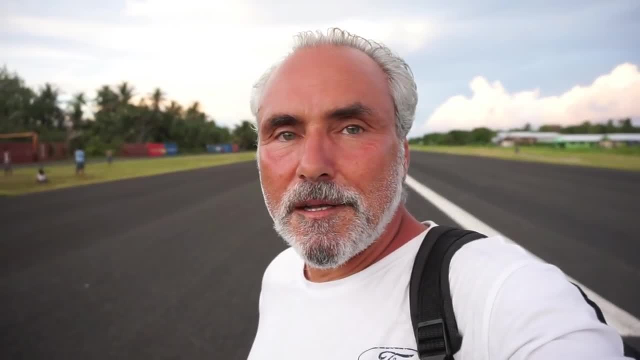 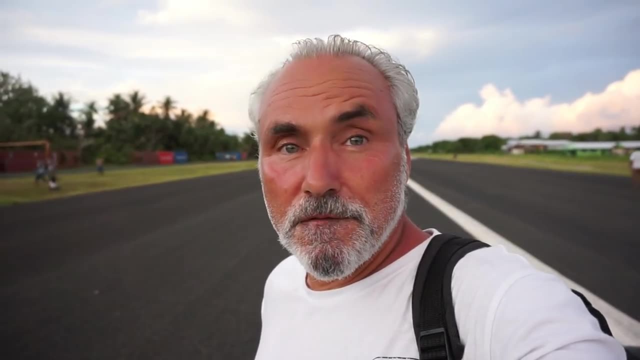 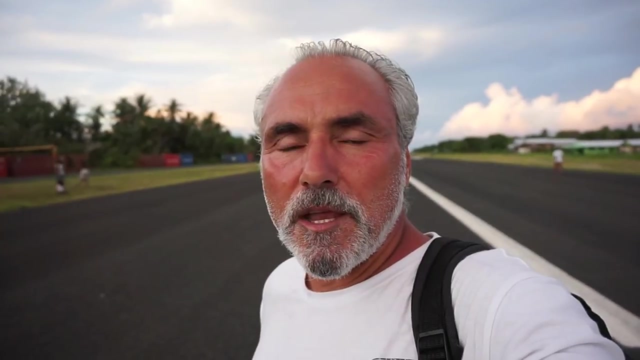 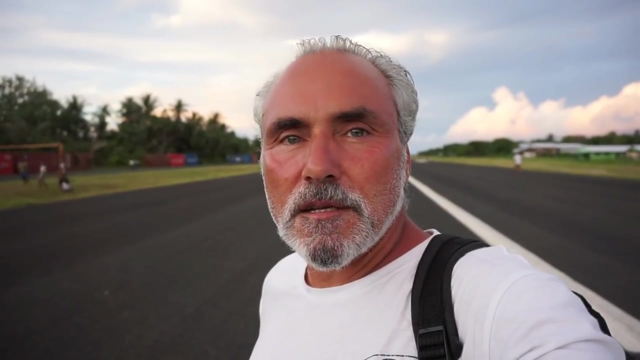 and here's another interesting fact: over 65 percent of the three thousand or so people they visit the country of Tuvalu per year are contractors that come here to work on different projects or they come here on business. Only about 20% of the people visiting Tuvalu are tourists. the rest are just simple Tuvalu. 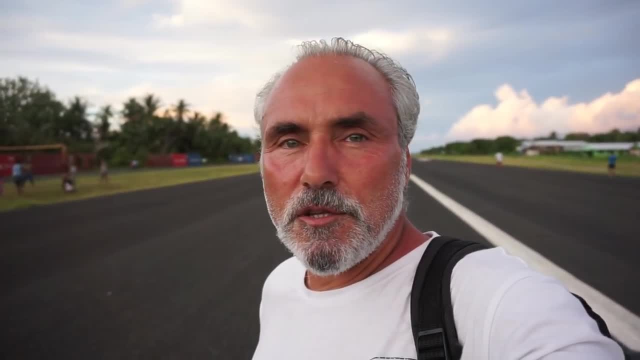 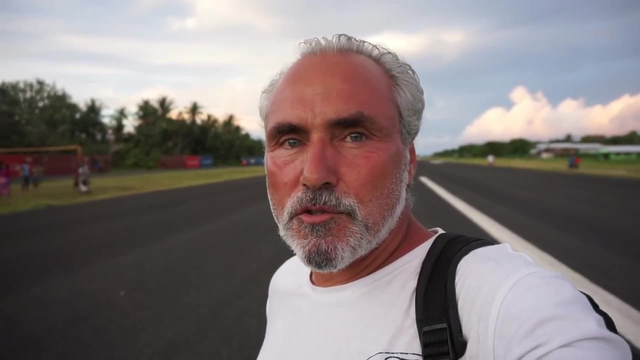 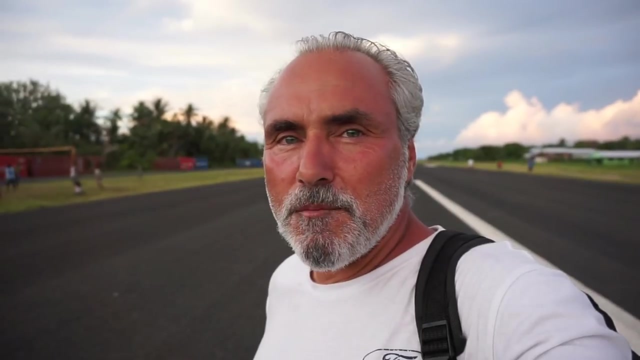 residents or citizens that return to the country to visit from New Zealand or other areas around the globe. Now, if you're one of the tourists- one of the 600 or so tourists that visit this country per year- a lot of people will come to you and they will be coming to you all the time. 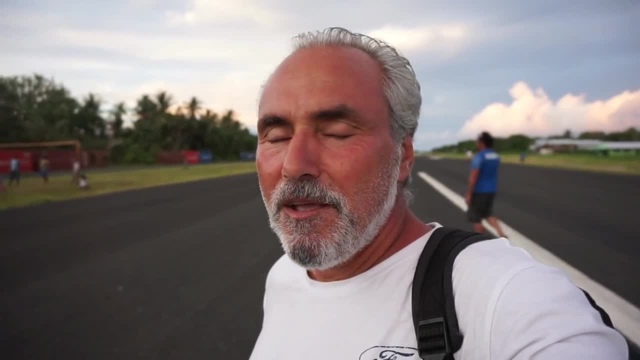 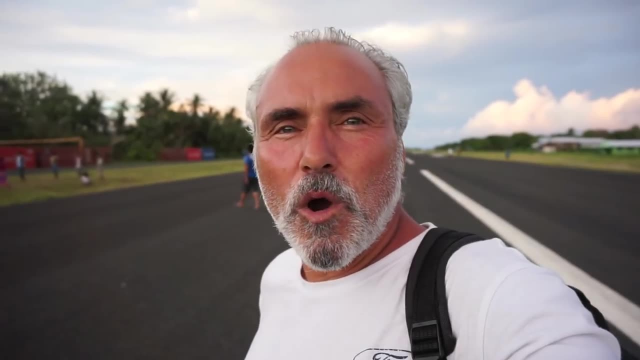 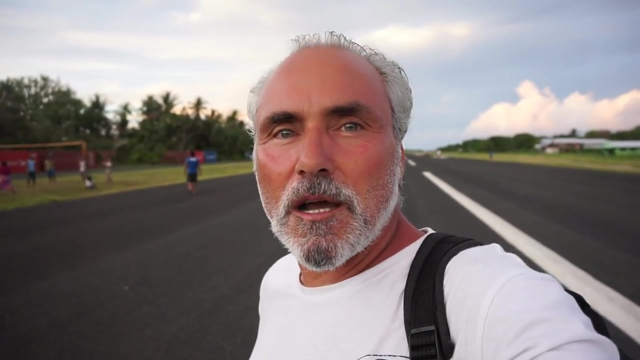 The first question they're going to ask is: where are you from? So you're going to tell them where you're from, and the second question, without a doubt it will be: why are you here? They're very, very curious why somebody would come so far away to such a small country. 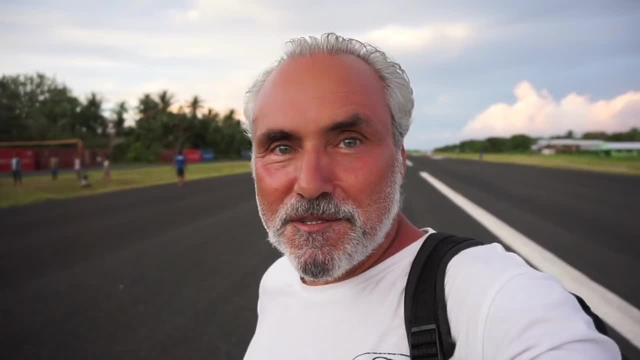 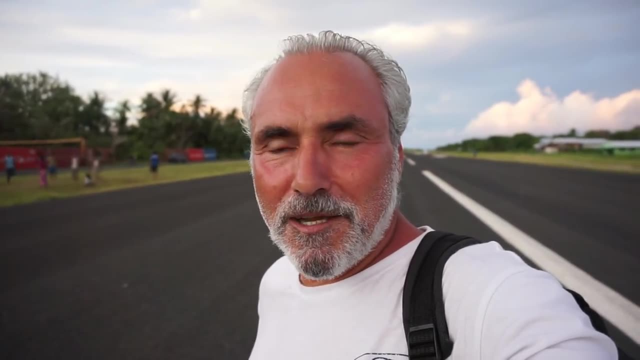 And the third question will be: how long are you staying? If you say I'm staying for a week, you really are going to stay for a week because you have no choice. There are only two flights a week out of Tuvalu. They're going to look at you and they're going to say: what are you going? 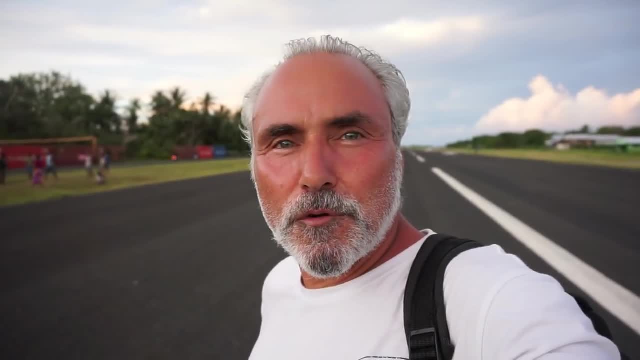 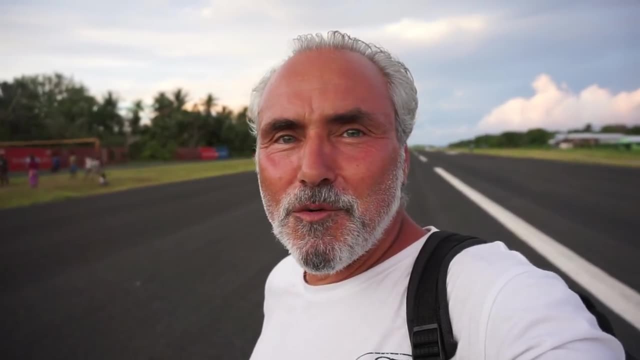 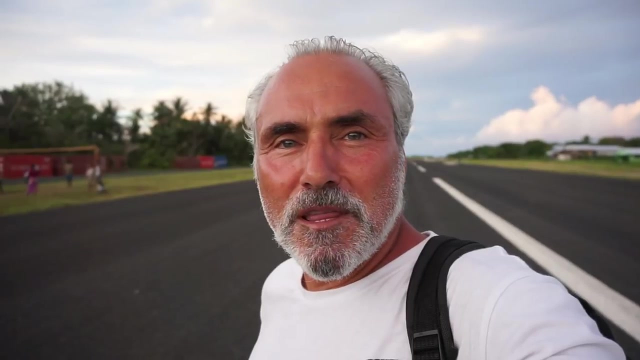 to do here. They're very, very curious where you're from. why are you here, how long you're going to stay? what are you going to do here? Because there is really nothing to do, which is not actually true, because it's a wonderful place, extremely friendly, and it's a memory that will last in your mind. 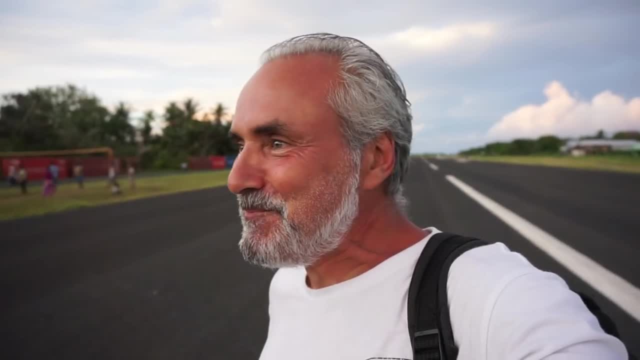 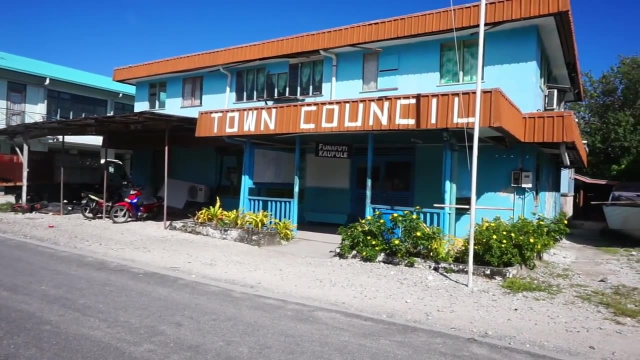 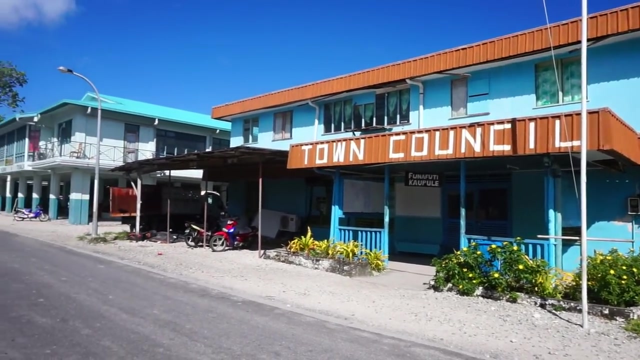 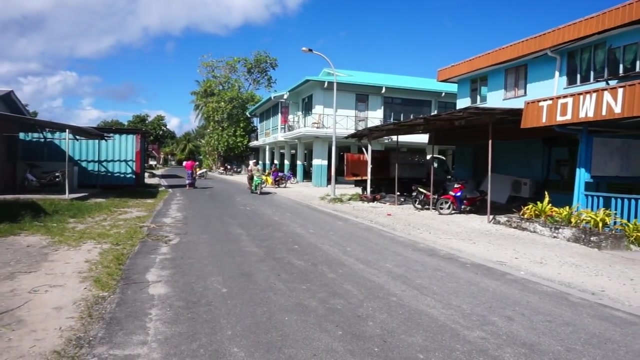 forever. Let's continue. And this building that you see right here is the city hall of Funafuti. right there It is closed. today it is Saturday, so it's rather quiet here. Here's a general view of the street in front of the city hall, which, incidentally, is: 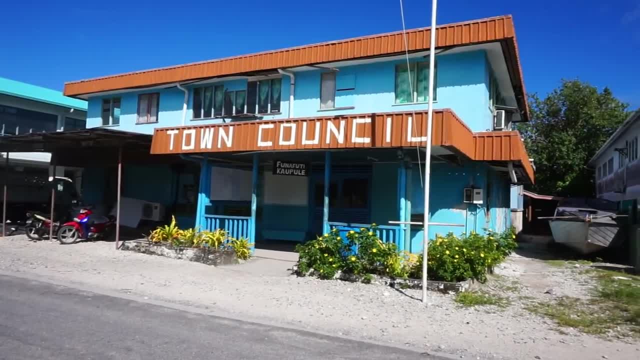 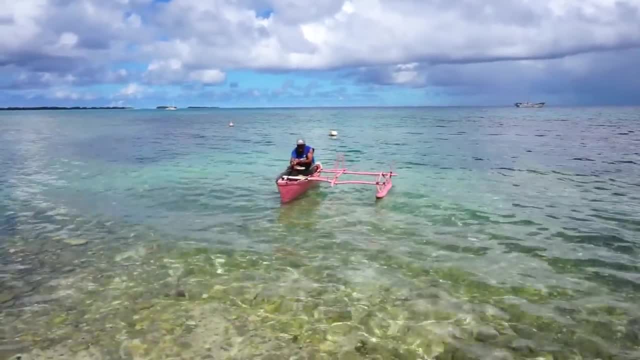 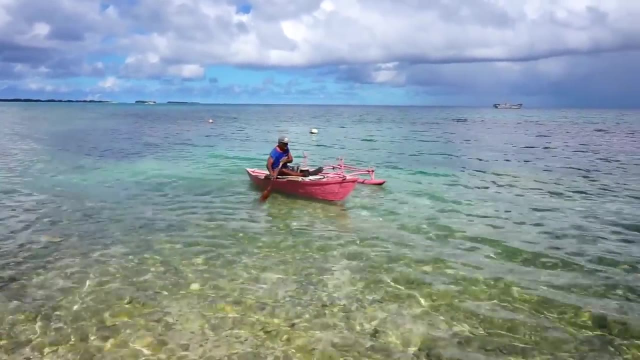 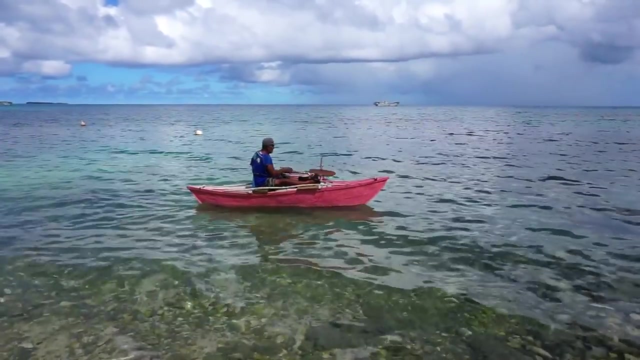 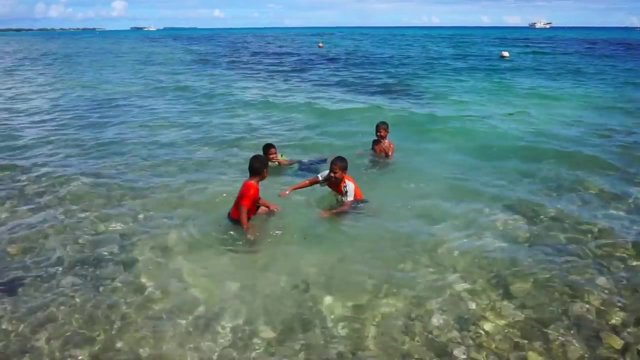 it is very close to the campus of the University of South Pacific And here's a view of the local fishermen Using a either a pink or a purple canoe for fishing. Look at that Here at the lagoon of Tuvalu. Hello. 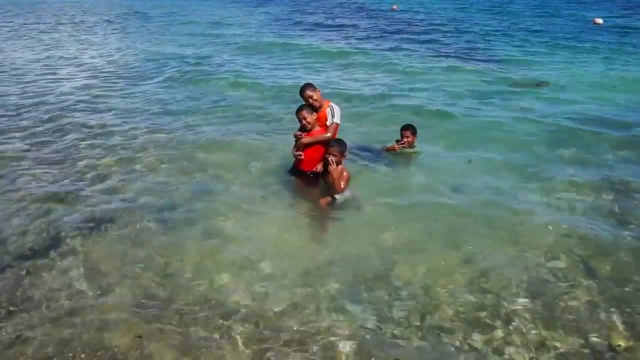 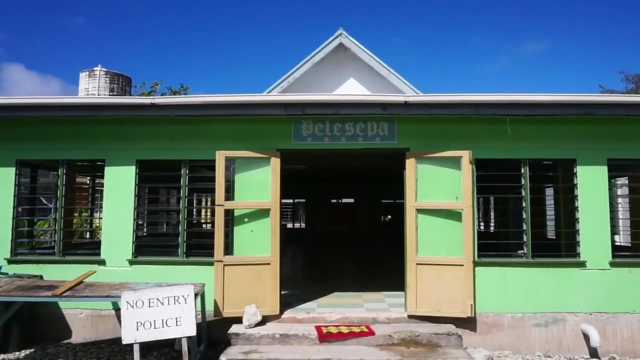 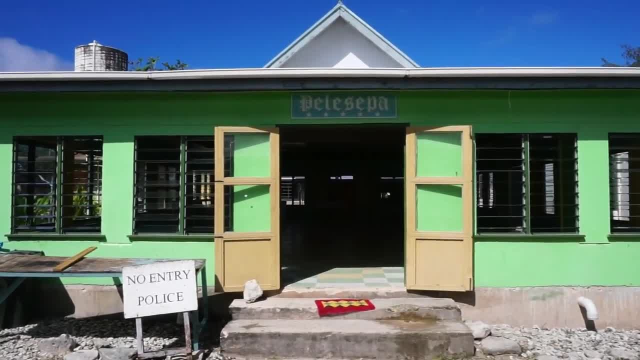 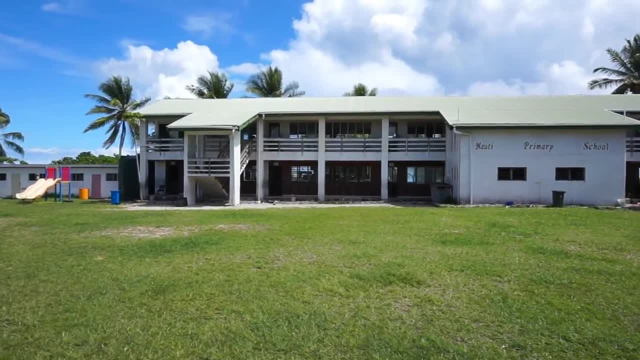 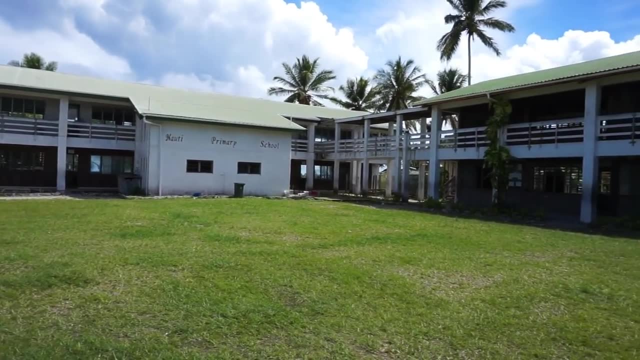 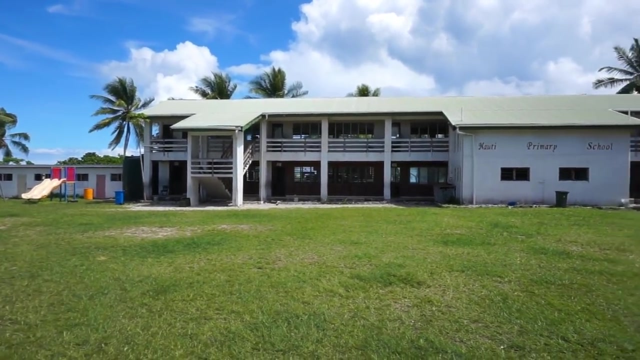 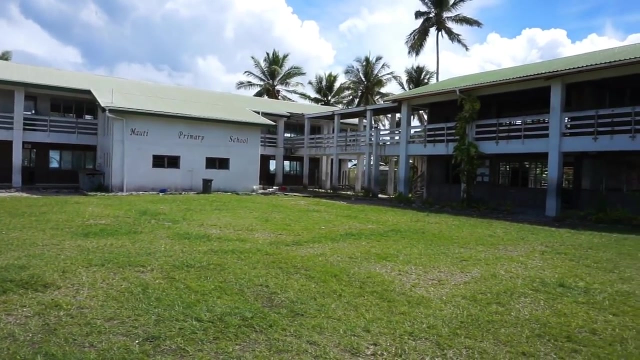 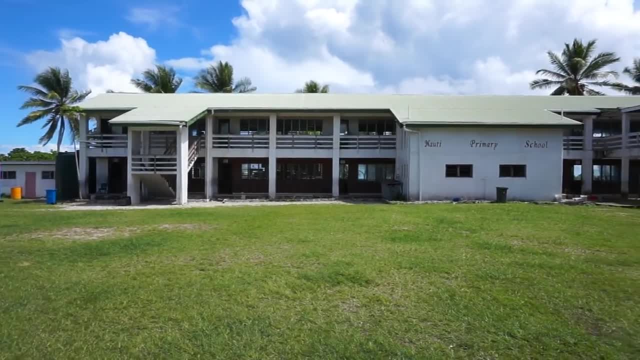 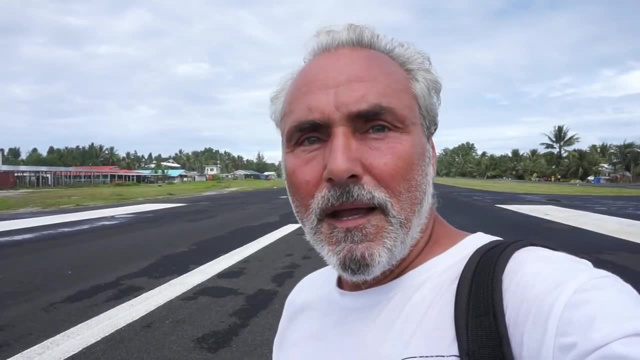 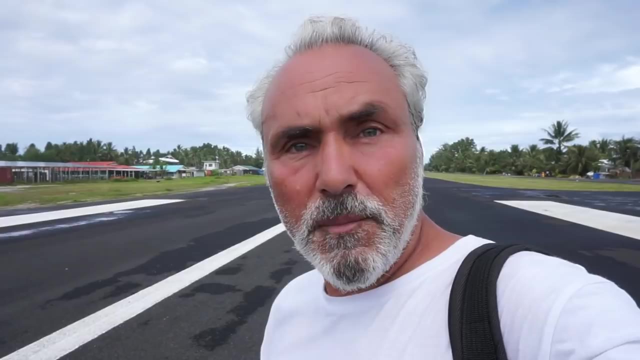 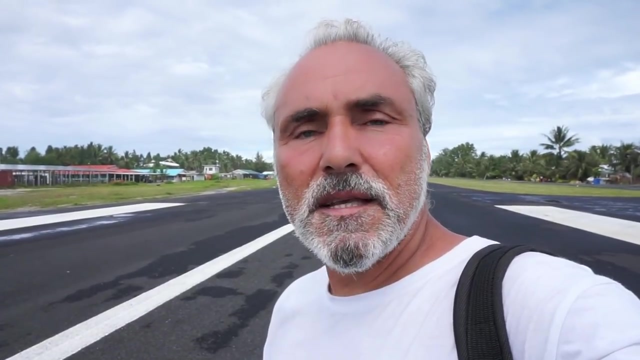 of the school which is right across the street from the University of South Pacific, the campus of the university. Now here's another fact: the highest point here in Tuvalu is 9 feet or 3 meters. that's correct. imagine living in a country where the widest point of your country is 600 meters. 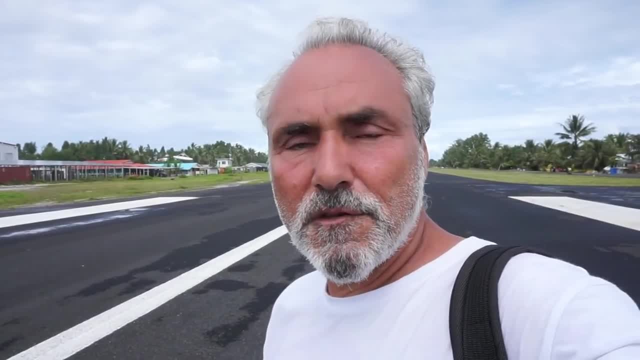 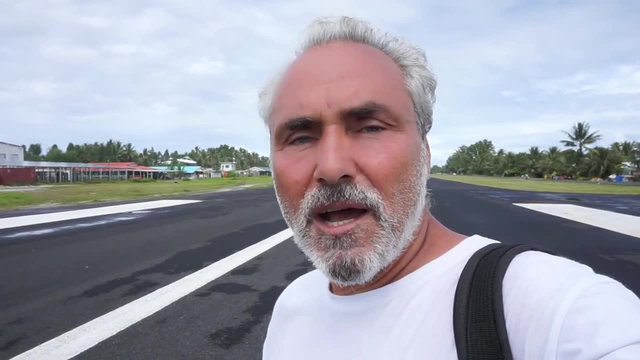 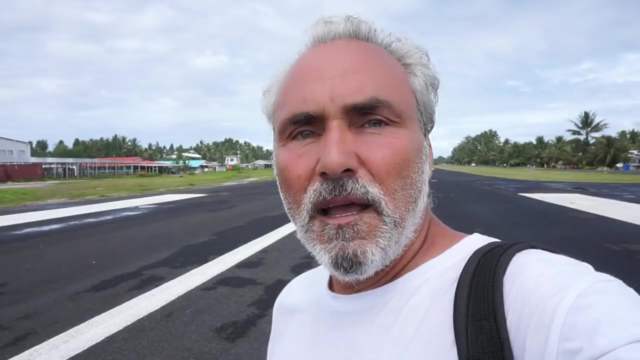 a third of a mile and the highest point from the surface of the water is 9 feet or 3 meters. also imagine that under your feet on the ground it is sand and coral. that's correct. There is no dirt, so there is nothing that you can do to grow vegetables here, for example. 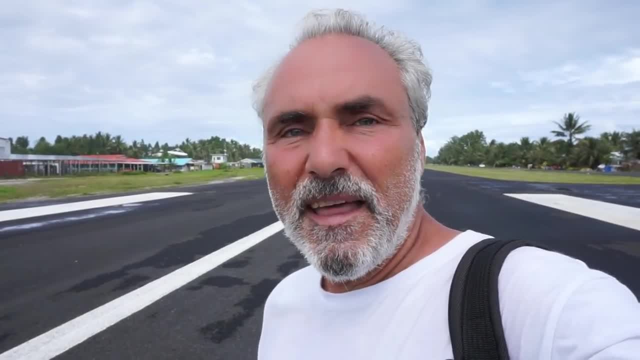 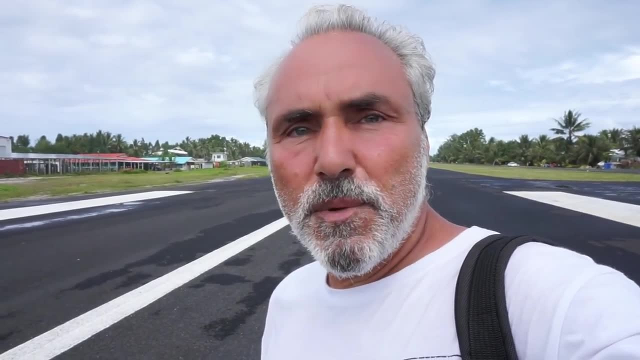 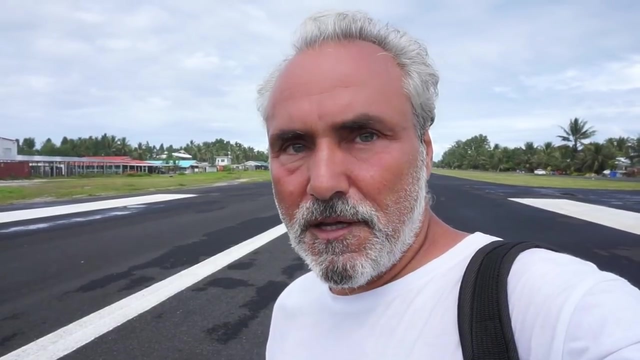 tomatoes or cucumbers. it's almost impossible. that makes the life here in Tuvalu very, very harsh, very difficult. that's why there are no sheep and cows here. there is nothing for them to eat. the only animals that they have are pigs, and lots of them. 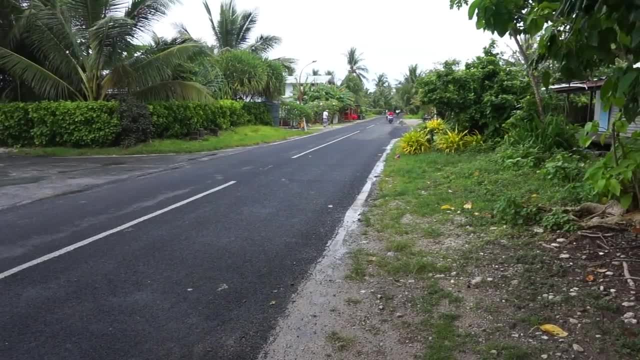 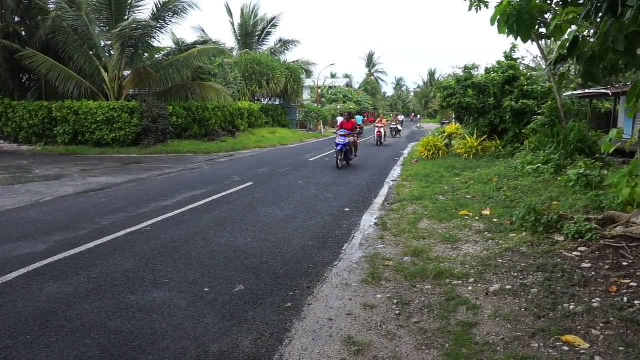 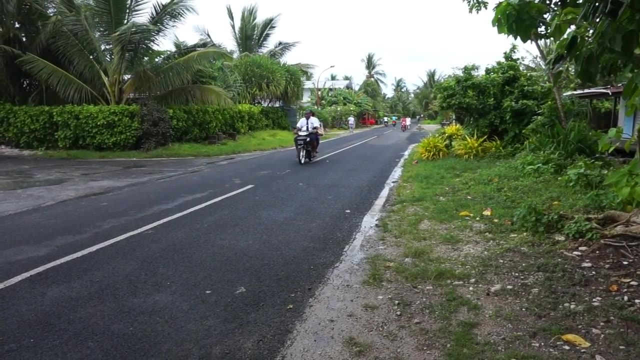 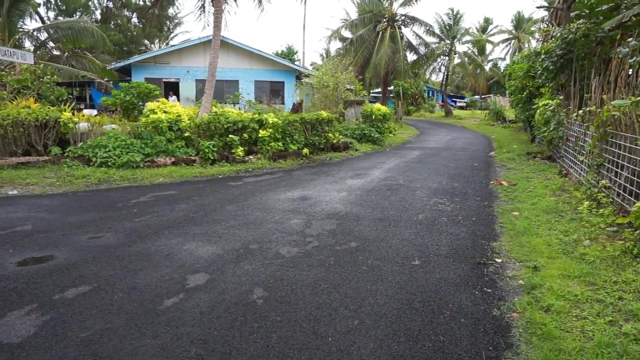 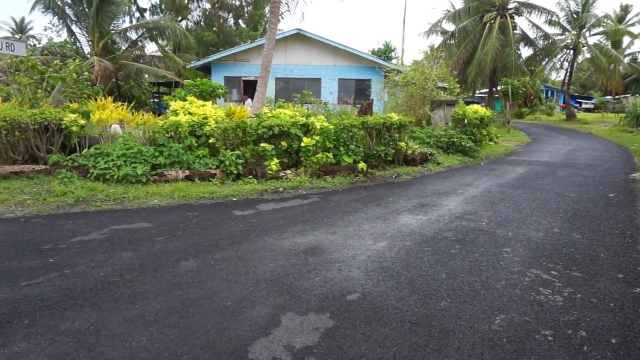 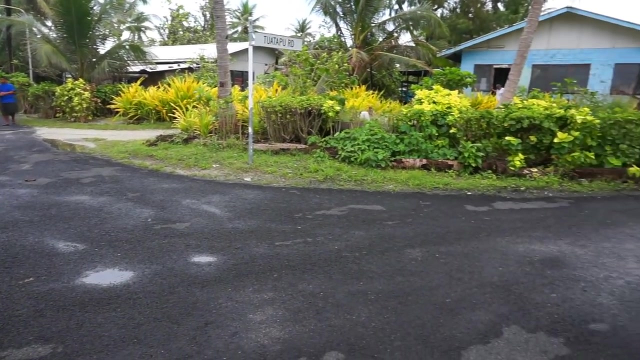 Now we are looking at a neighborhood road here which is thankfully not busy with motorbikes, and here attached to a mountain. so we are just having fun for a little while. and then, But about six years ago, Tuvalu had no paved roads to speak of. 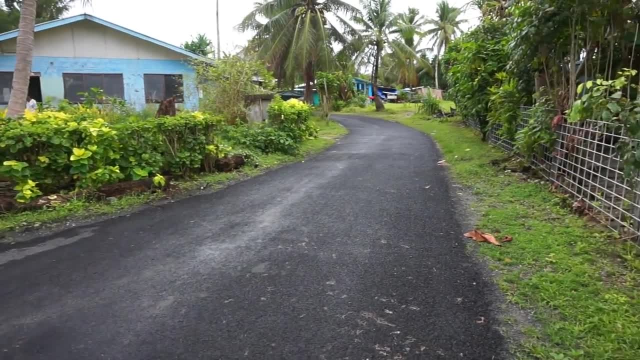 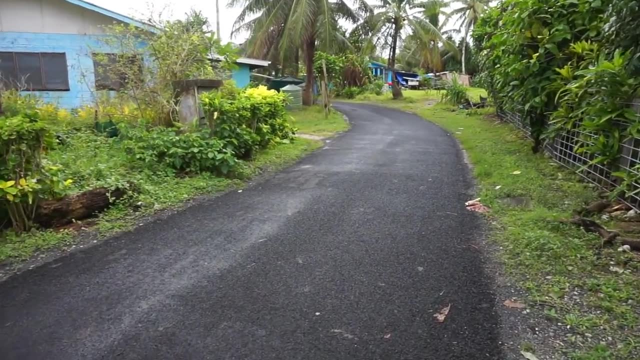 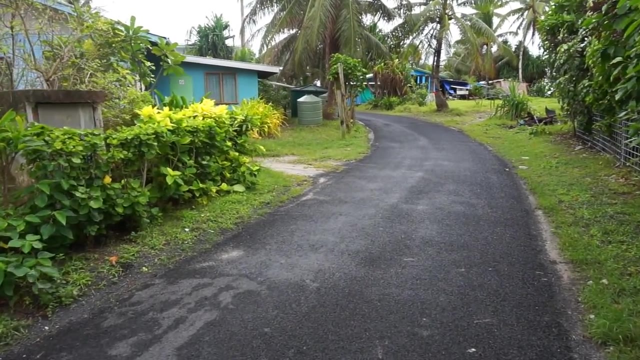 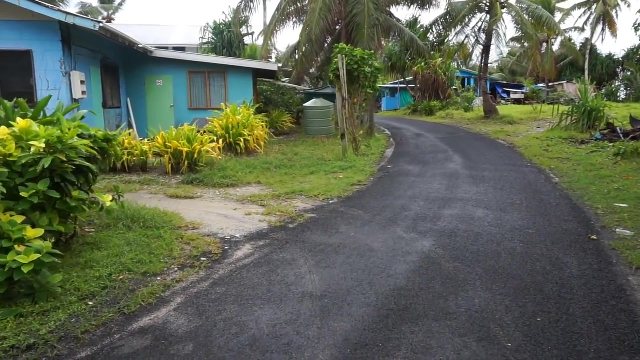 Now it's got about 10 kilometers of beautifully paved roads, brand new roads. Actually, you can see the condition of this one is perfect. Now what's happening here in the Central Pacific? in a lot of countries like the Solomon Islands, Vanuatu, Tuvalu and other places, there are three huge agencies that are being involved. 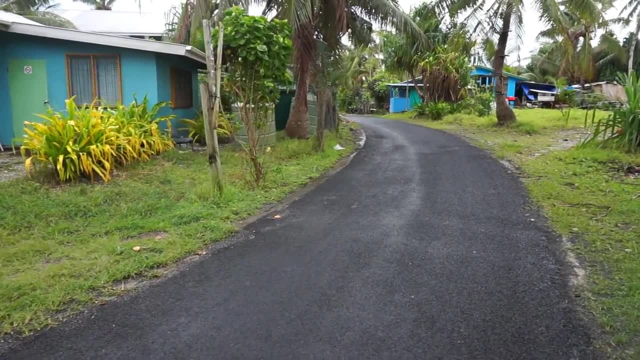 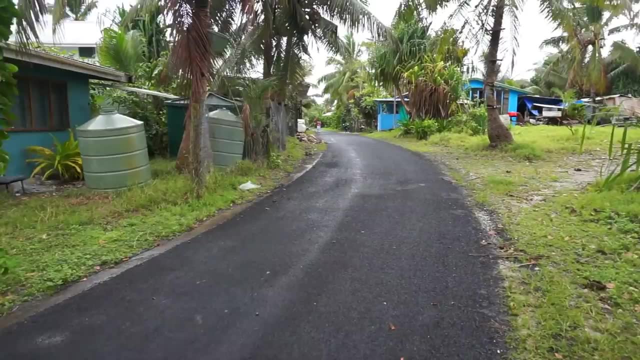 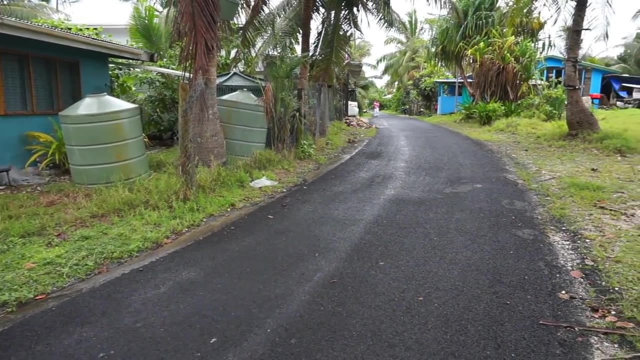 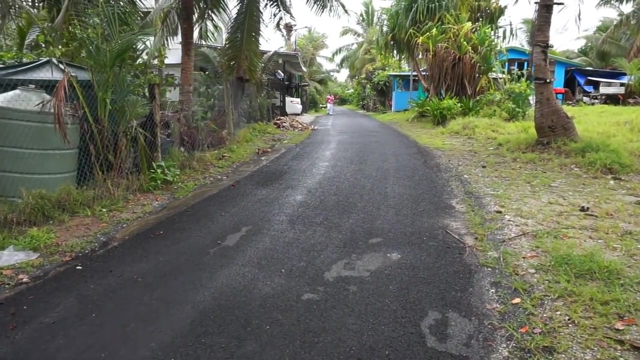 in improving the infrastructure of this less fortunate countries. One is by far the World Bank that finances these big projects at low interest rate. Second, secondly is the Australian Government, through AustraliaAid, In~~~. If you come to the Pacific, Central, South Pacific and Western Pacific, you will never. 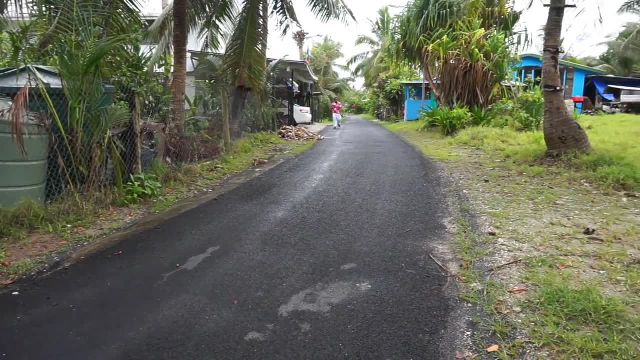 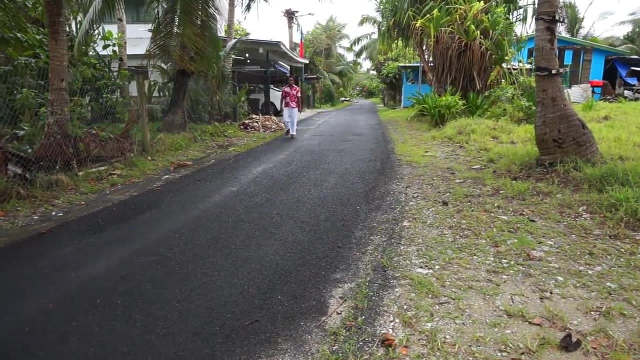 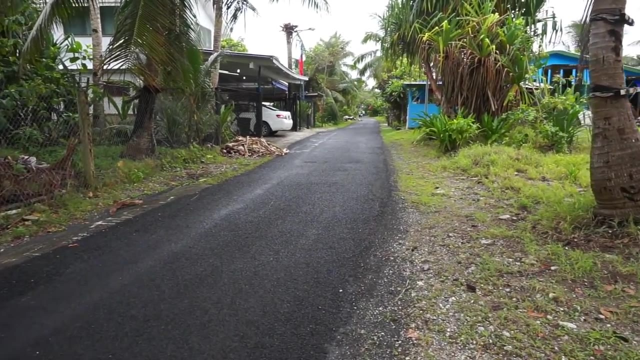 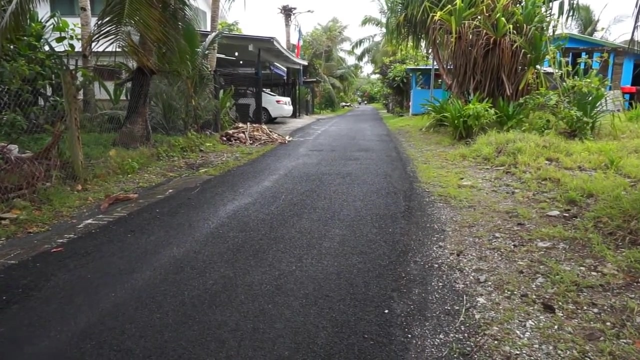 miss the signs From Australia, Aid that agency that donates the money for the infrastructure projects. And, lastly, the Government of New Zealand, who saw the road from Munda to Noro in the Western District of the Solomon Islands, the island of New Georgia, 15 miles of it paved. 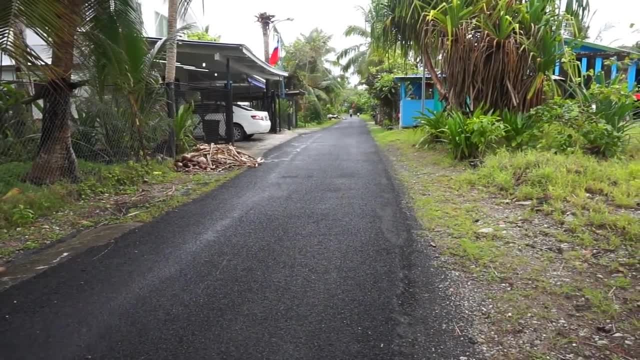 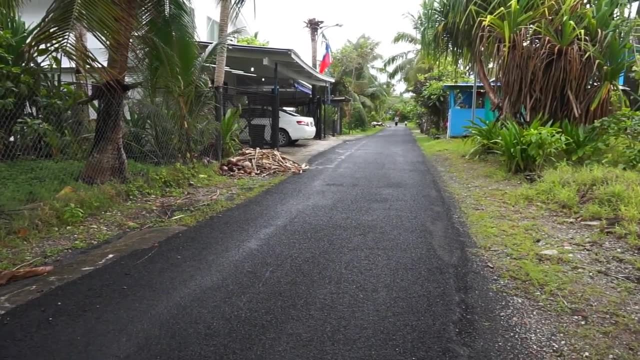 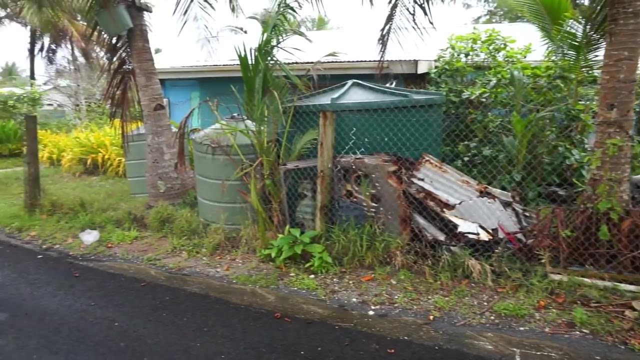 beautifully by the New Zealanders, including the runway in Munda in the Solomon Islands. So these three agencies are very heavily involved in improving the infrastructure of these less fortunate countries and islands. Here's a good example here that you can see About 10 kilometres apart. 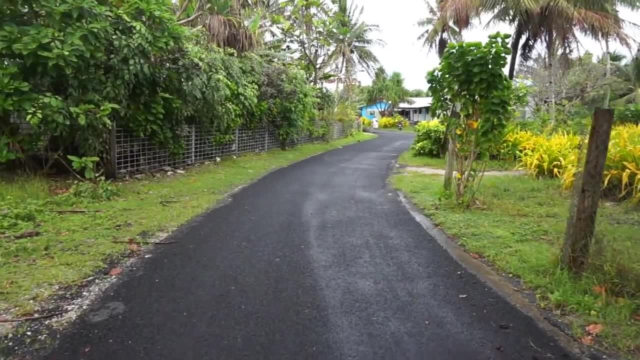 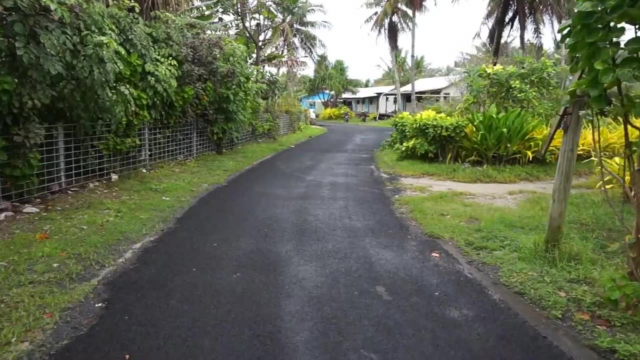 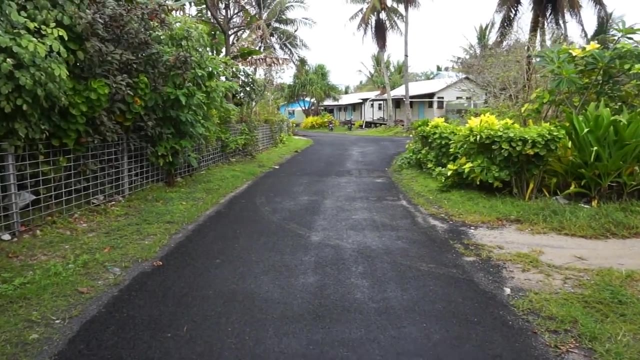 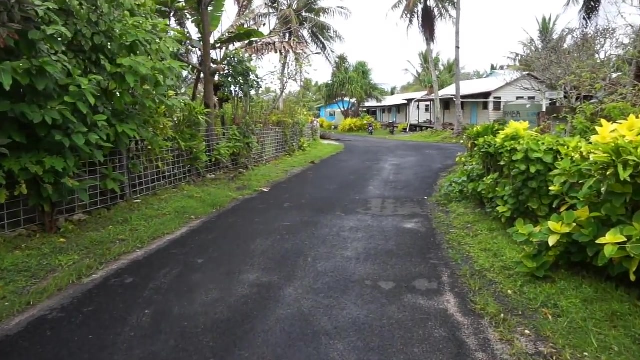 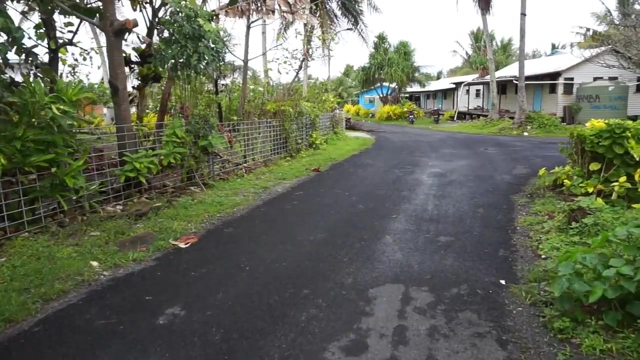 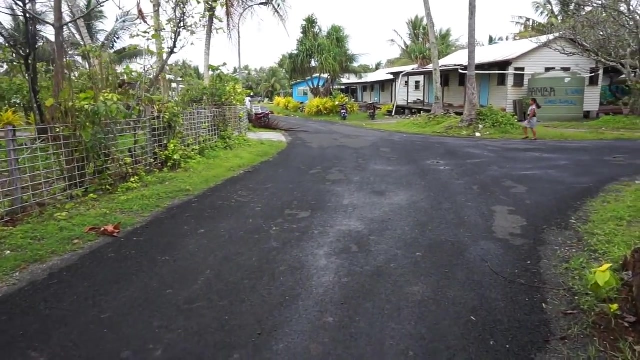 Paved road that tremendously improved the lifestyle of Tuvalu. Now there are two other entities that you will see participating, And one is the Chinese government as well. You will see some huge projects where the Chinese are involved here as well. Unfortunately, you're not going to see anything about the American government or the Russians. 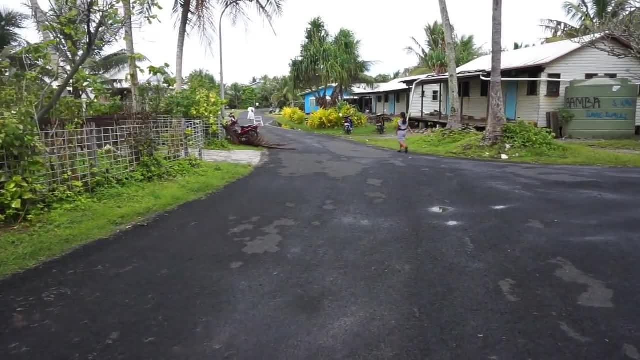 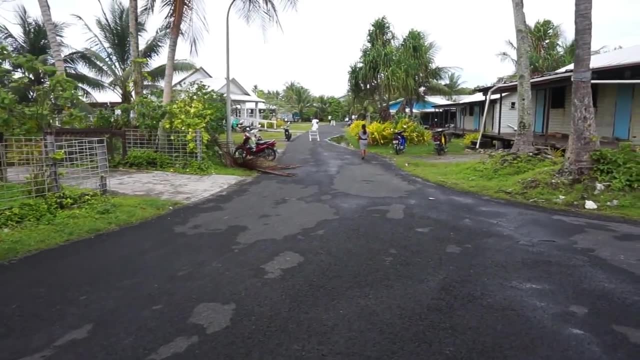 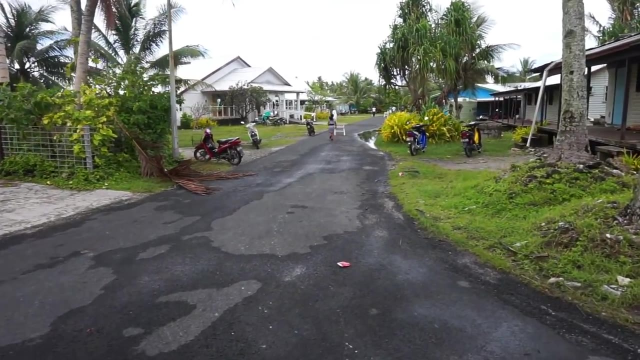 And here's another view of the road. It is Sunday. You can see people going to church, which is to the left of the frame. You can imagine this road here about six years ago- A dirt road. Imagine how dusty it must have been. 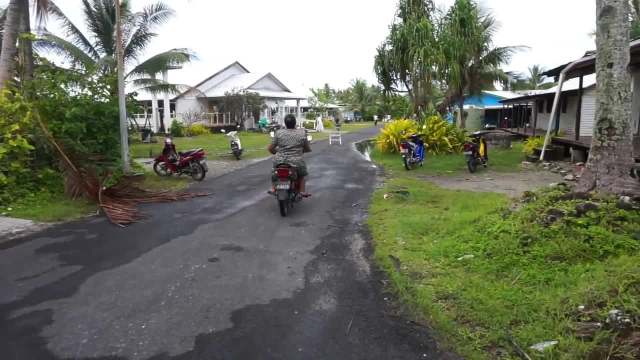 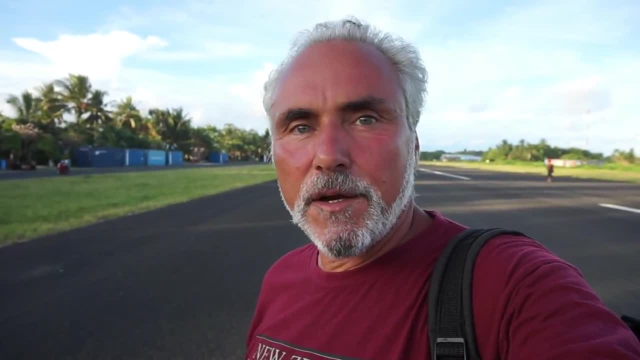 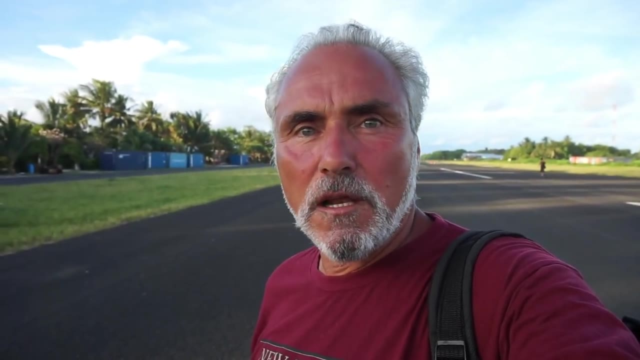 It's very dusty. And look at the difference now. If you put together all the islands and the reefs here in Tuvalu, you will get a landmass of about 15 square miles, or about 26 square kilometres. Here's another fact. 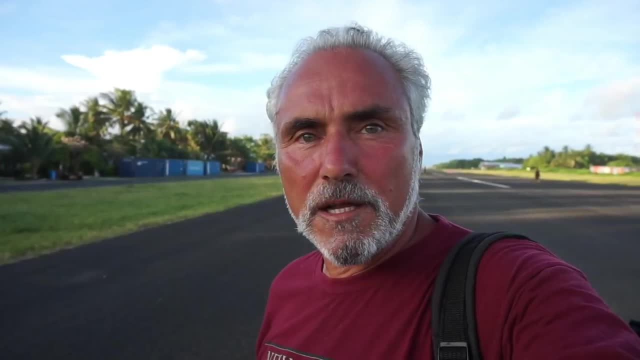 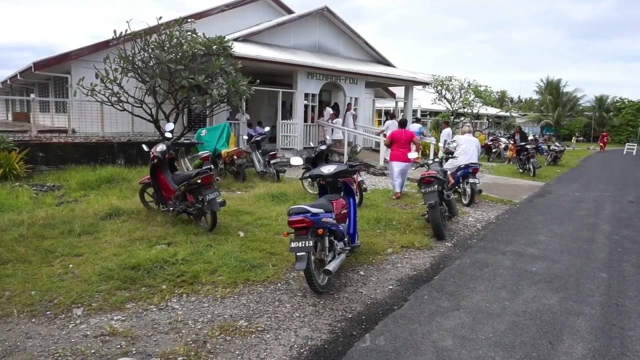 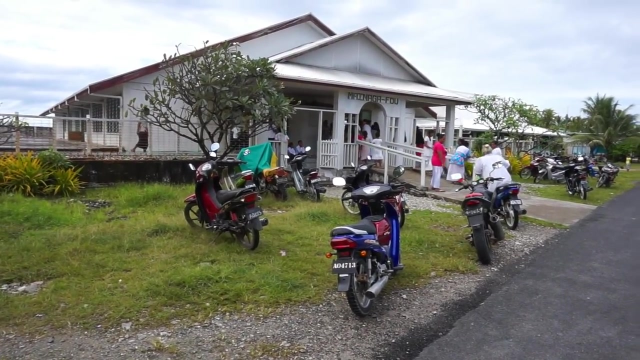 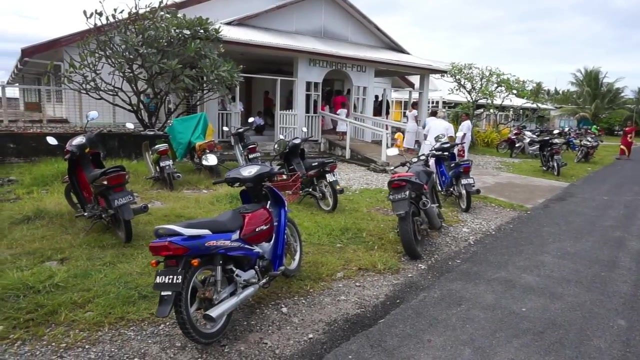 One of the largest sources of revenue for the government here in Tuvalu is selling stamps, Yeah, stamps. And here's another church, another Methodist church. It is also called the Church of Tuvalu. It is Sunday morning. You can see the motorbikes parked. 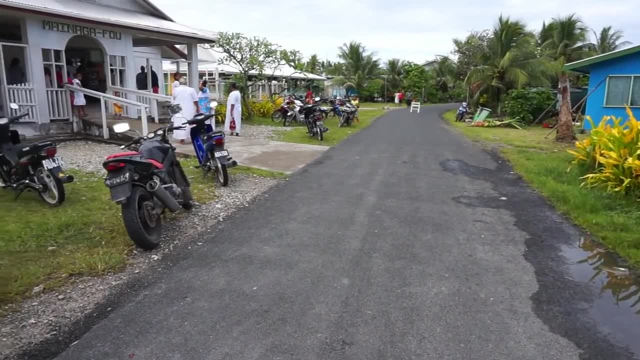 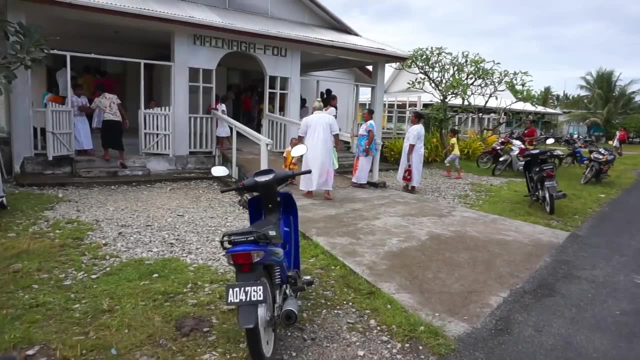 What do you do here? on Sunday? They close down the road to traffic. Let's go a little closer so you can get an idea of what it looks like. This is a traditional church. This is a traditional church. It's a traditional Tuvalu church. 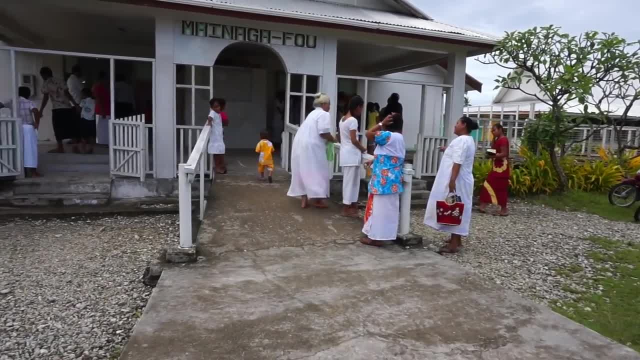 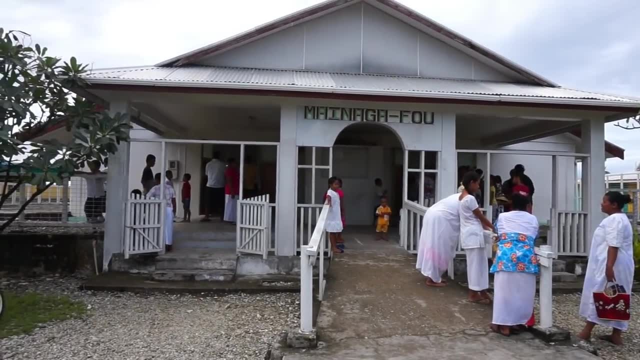 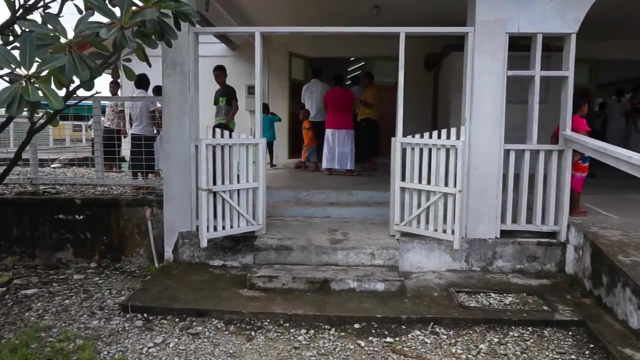 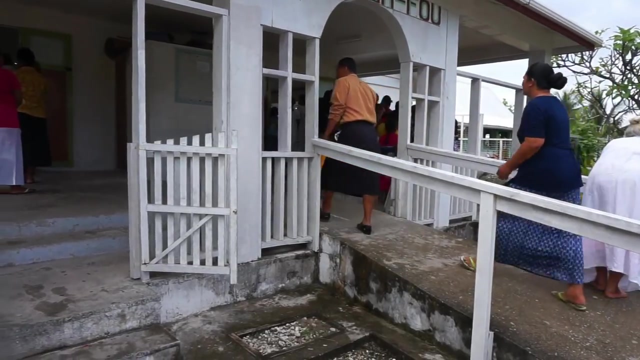 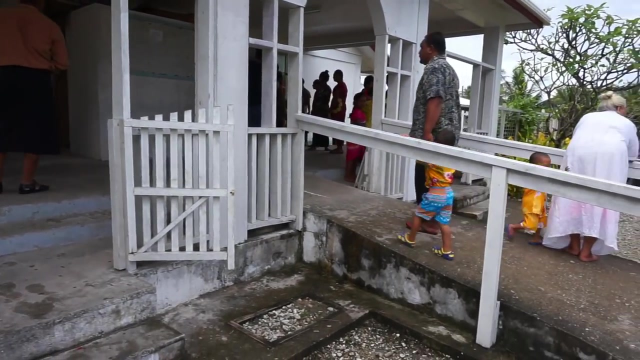 You can see the ladies dressed for church. service just started a few minutes ago. Now I want to show you something that we have not seen anywhere in the Pacific as yet. What happened happens. here is some of the people coming to church carry fans. here's the. 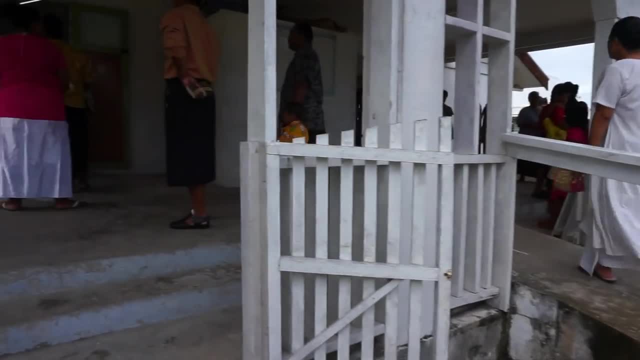 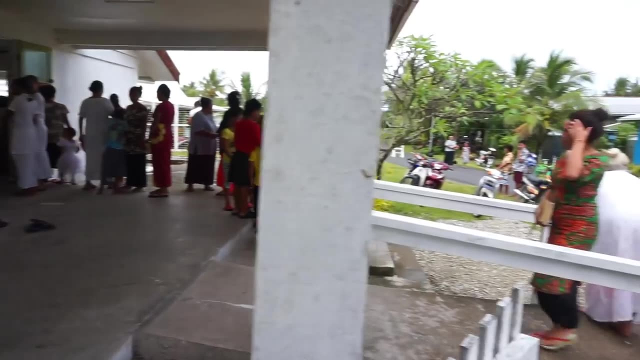 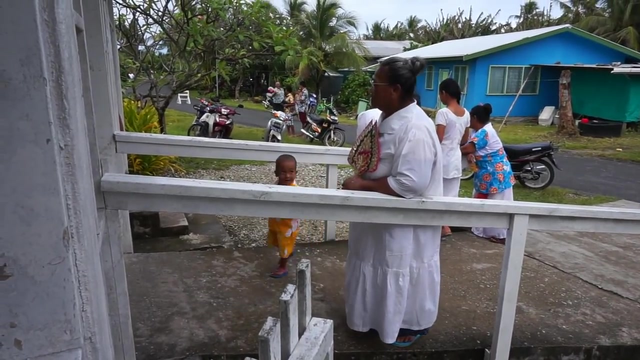 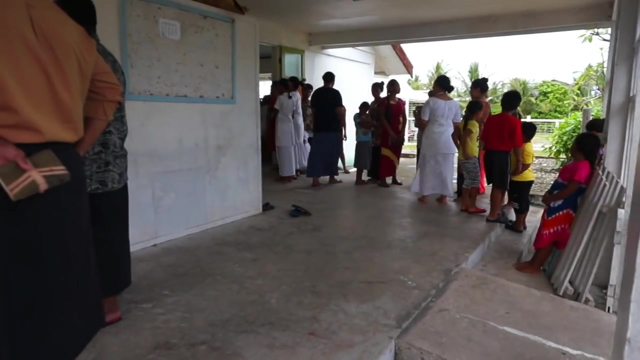 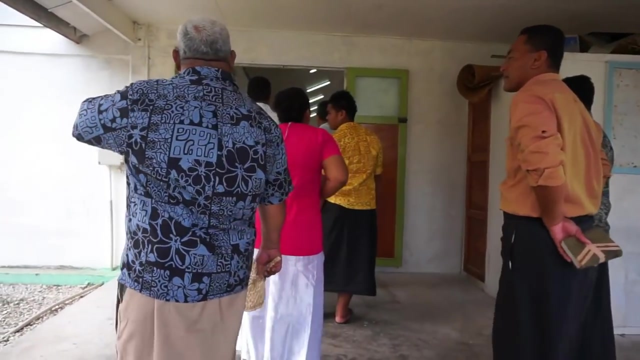 lady. this is holding a fan that's going, so you can see the fan right there and people come here holding you can see more here. look at this holding elaborate fans. it gets hot inside the building but the fan carrying you can see this gentleman over here as well. he's holding a fan right there, so you can see fans. 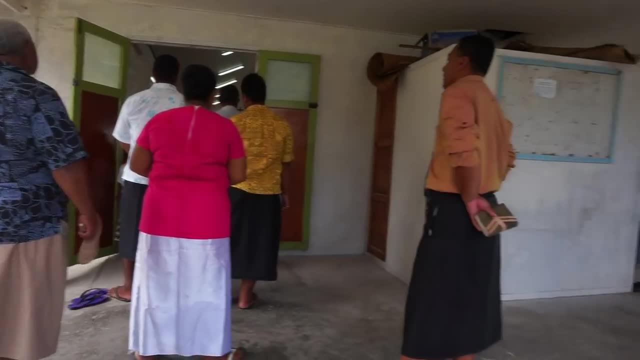 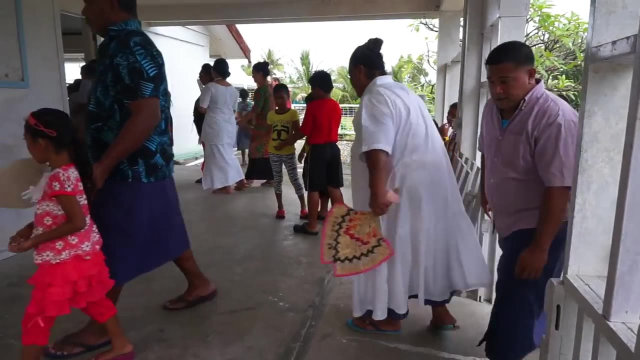 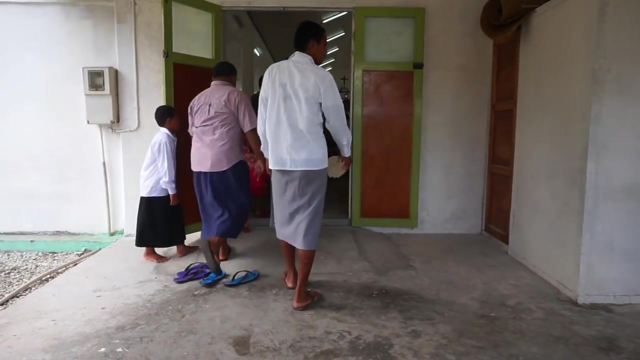 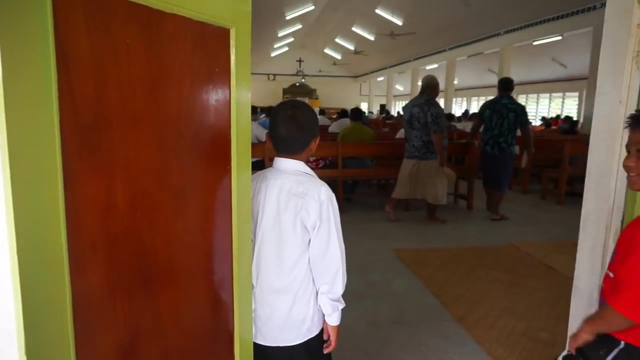 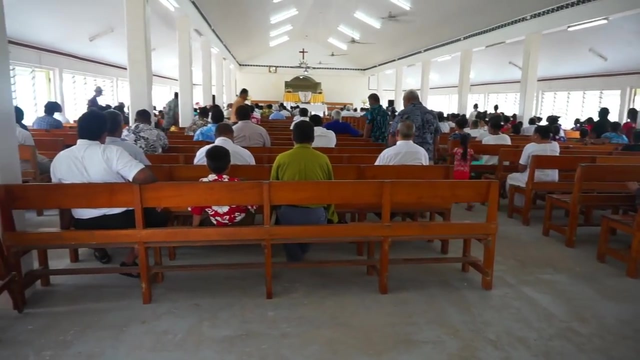 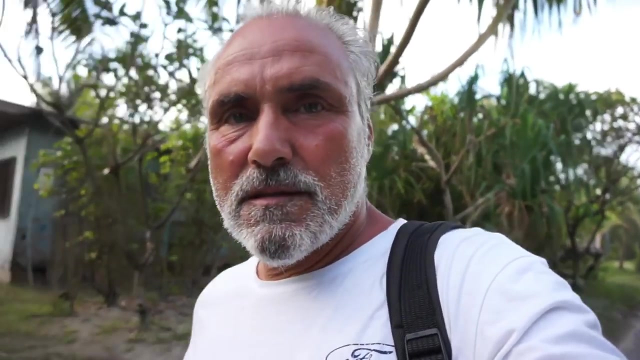 here of all sorts of different kinds, decorated beautifully. there's more people coming. you can see this man here with a fan. you can see the lady with a fan here right there. let's go inside for a moment. I'm not just south of the runway and I'm walking towards the southern direction. 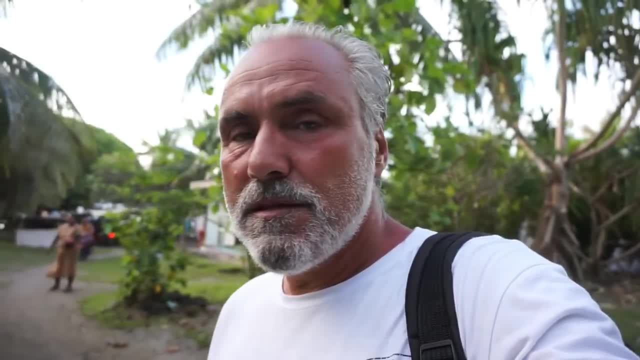 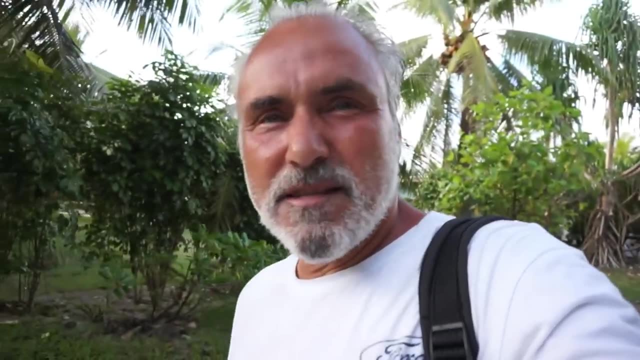 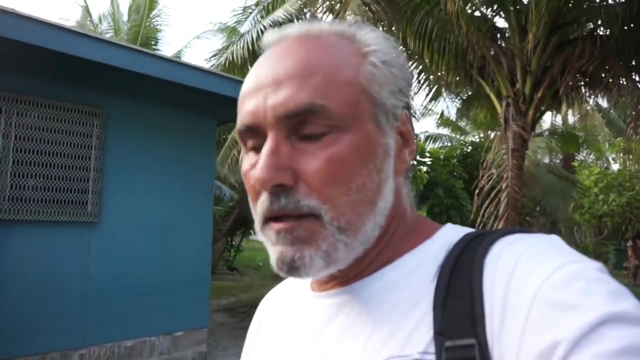 to my left, in about 20 meters distance, I can hear the waves crashing onto the eastern coast of Tuvalu. to my right, I can see the water as well. the width of the country at this point, where I'm right now, is 15 meters 150 feet, so imagine living in a. 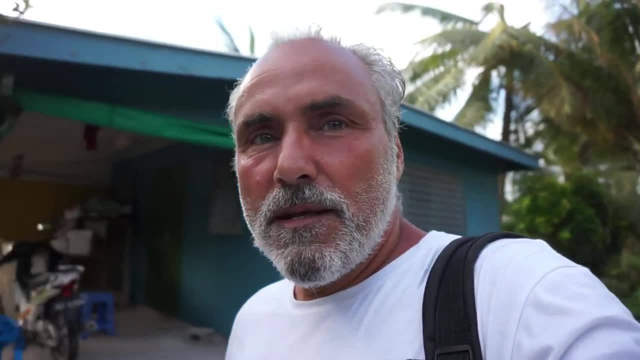 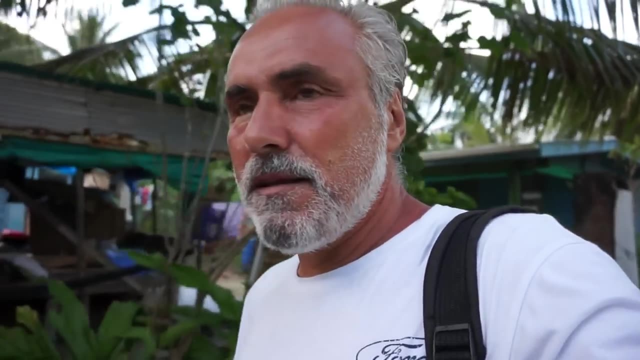 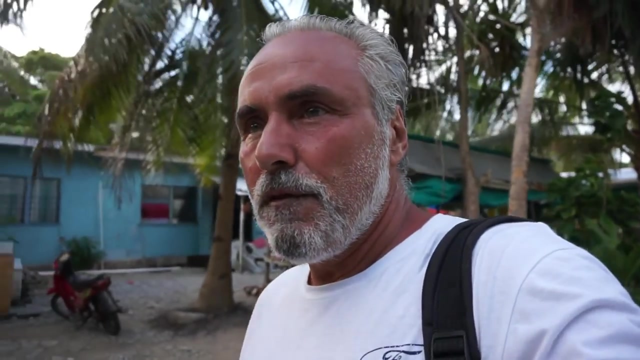 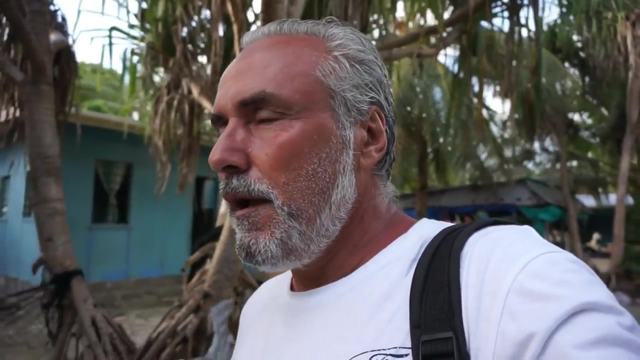 country where, in certain places, the width of your country is 150 feet. it is absolutely hard to imagine, isn't it? this is reality here. but the people of Tuvalu, they have to live here, they have to do their best. in this small country was such harsh environment and hardly any resources to. 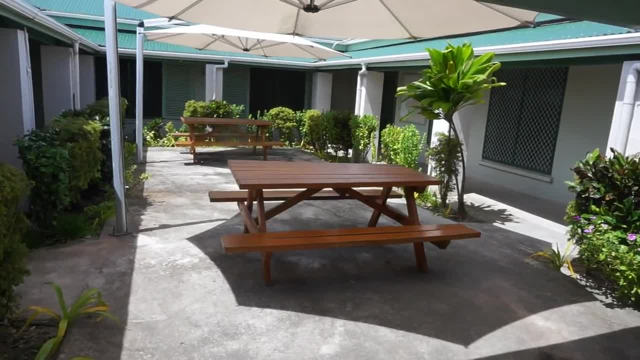 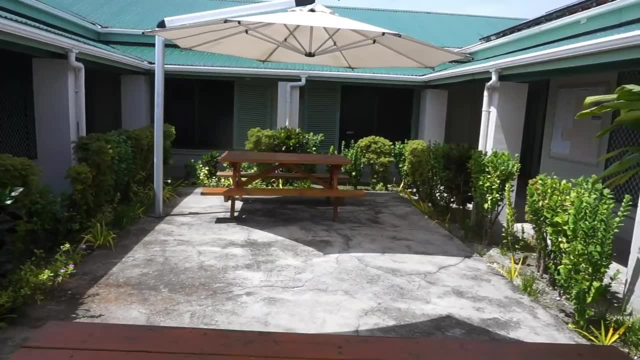 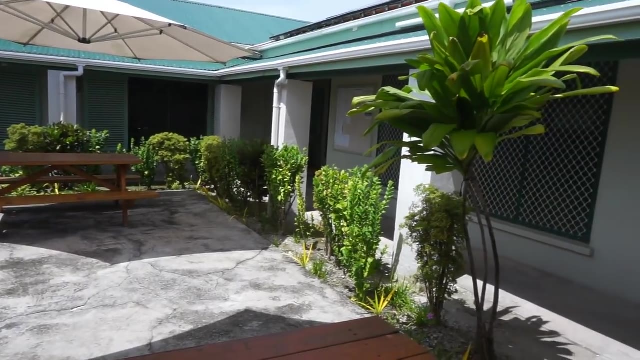 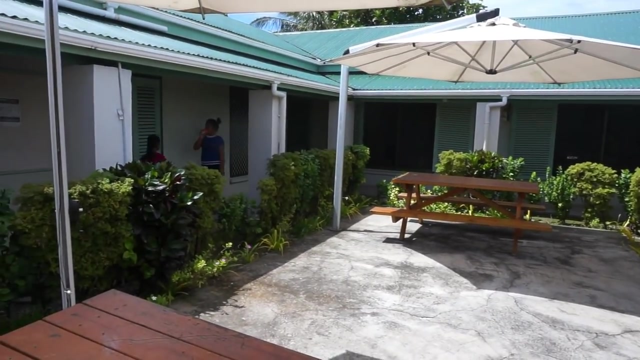 live with and to exploit. and here's the campus of the University of South Pacific here in Tuvalu: very small campus for three hundred students. very small campus for three hundred students. Of course, the University of South Pacific has campuses all over the South Pacific and it is co-owned by 12 countries. 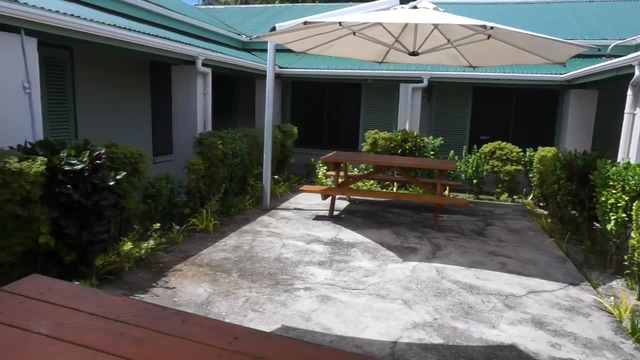 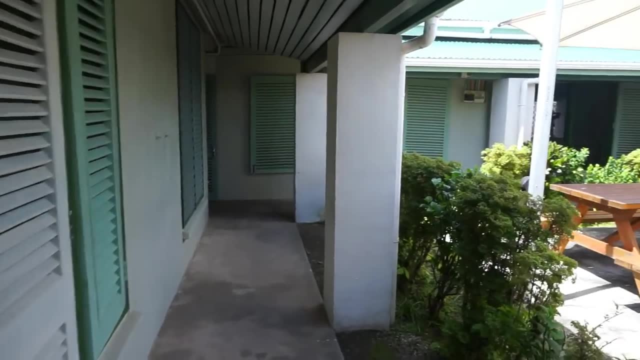 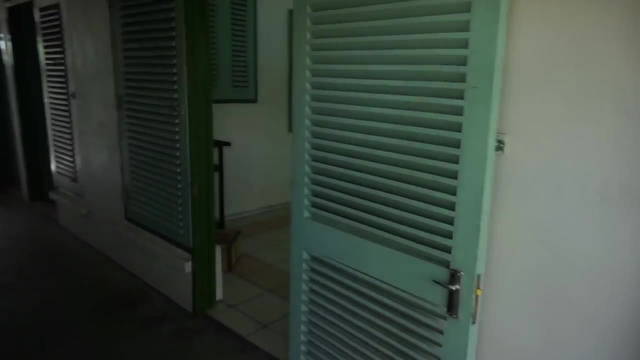 We've seen campuses in Tonga and Fiji. Let's go inside a couple of the rooms. It is a very small place, but it's beautiful nevertheless, for only 300 students here in Tuvalu that attend the university. Here is one of the large classrooms. 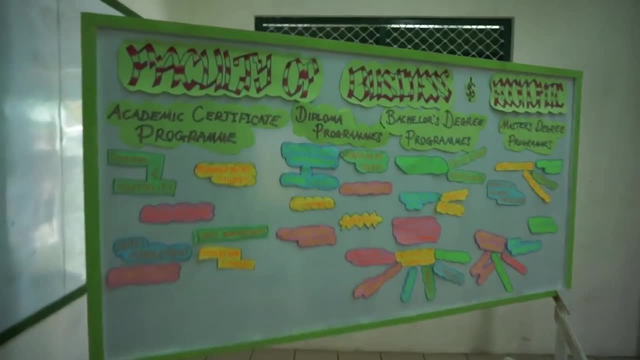 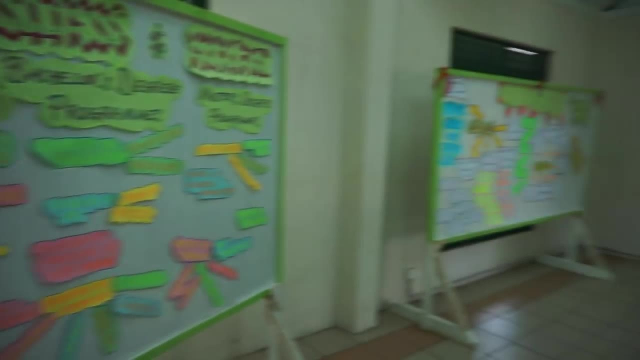 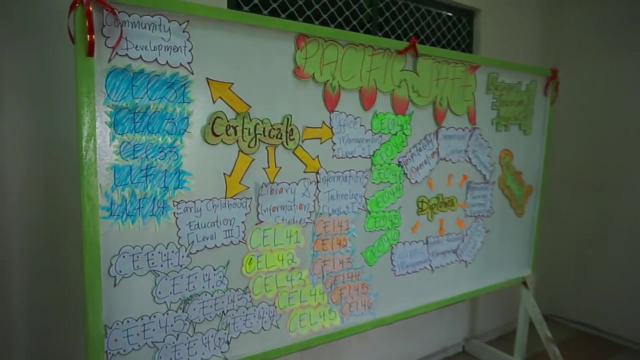 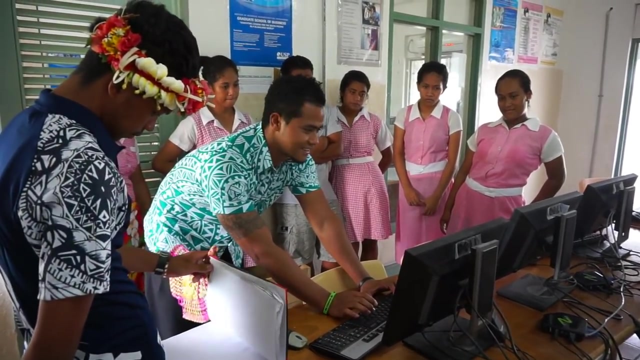 You can see the different disciplines here: different diplomas, management, business. Now there is an open house today. you can see some of the students getting ready to dance outside And this is the computer lab Here Here at the campus in Funafuti. 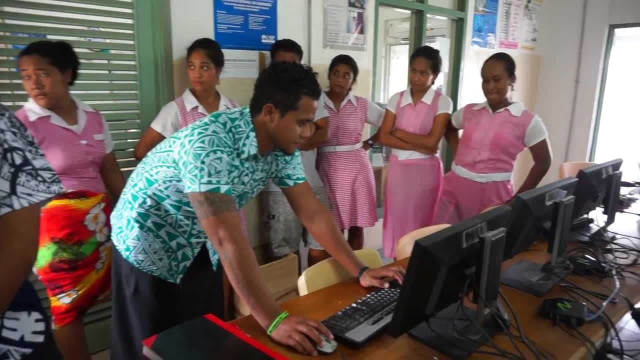 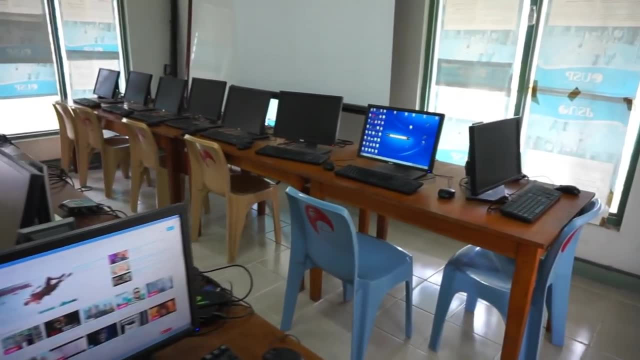 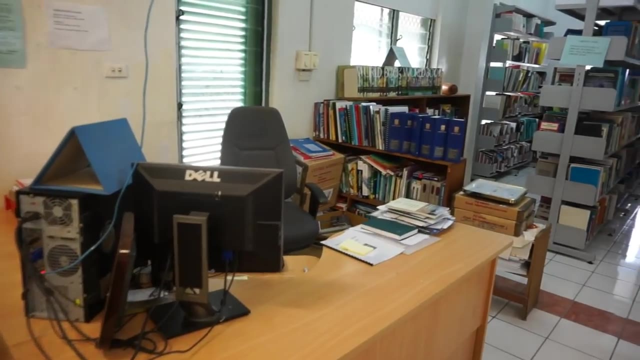 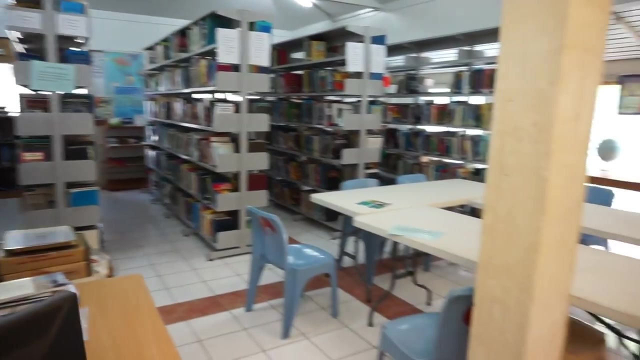 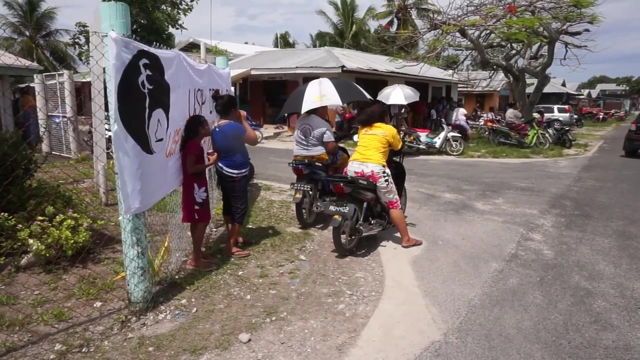 And here is a member of the staff showing to them the computer facilities that you see here. Here is the computer lab And here is a view of the library facilities here at the University of South Pacific: Books on the shelves, Computer equipment. Now we just looked at the campus of the University of South Pacific, which is to my left. 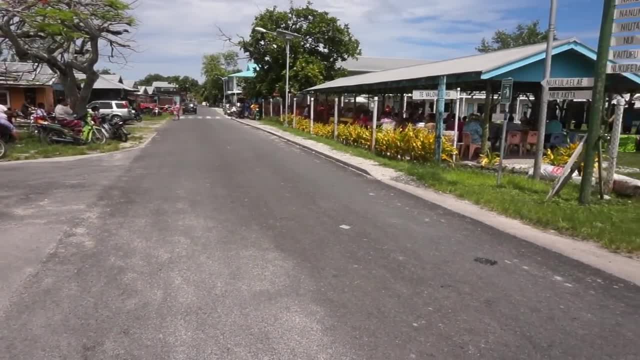 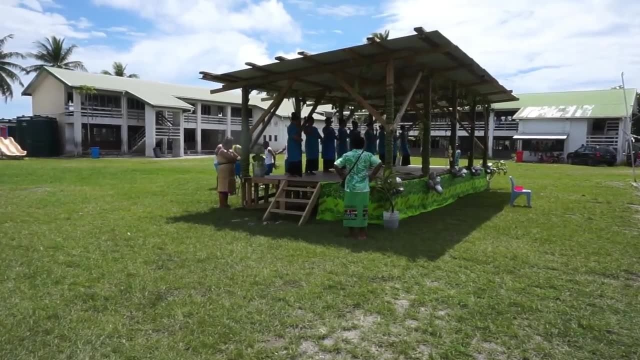 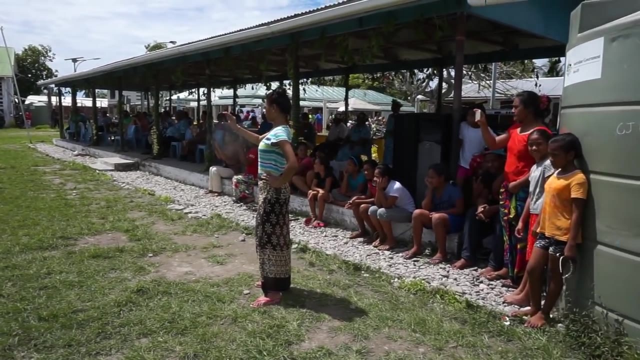 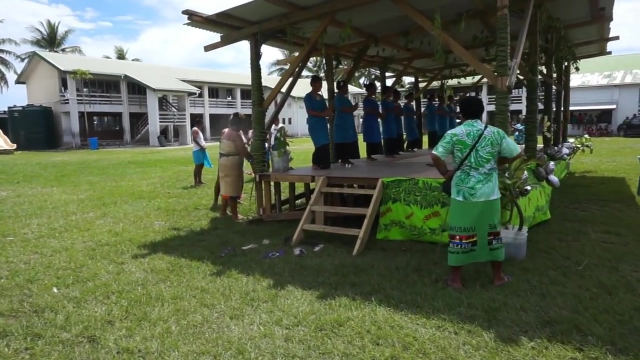 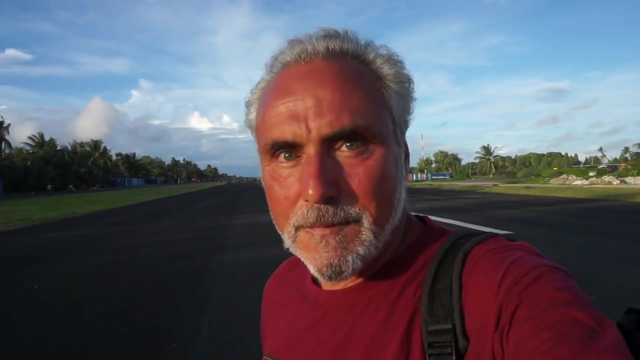 And there is an open house today And right across the campus there is dancing by the students. Now we just looked at the campus of the University of South Pacific And right across the campus there is dancing by the students. Now let's see if I can get this fact straight without making a mistake. 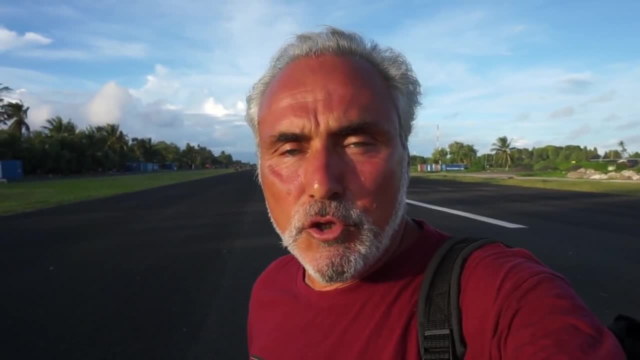 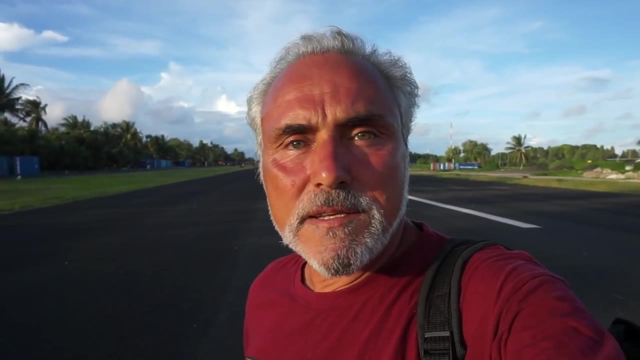 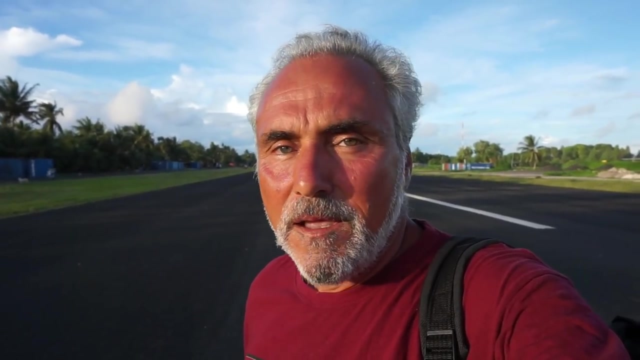 When Victoria was Queen of England in 1892, a single colony was formed here in the Pacific that combined the Gilbert Islands, which are known today as the Republic of Kiribati or Kiribati, and the Ellis Islands, which are known today as Tuvalu. 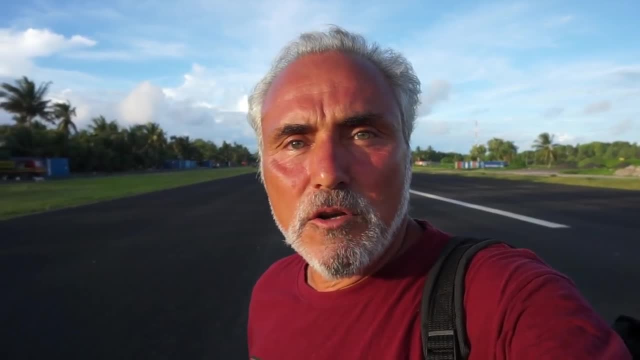 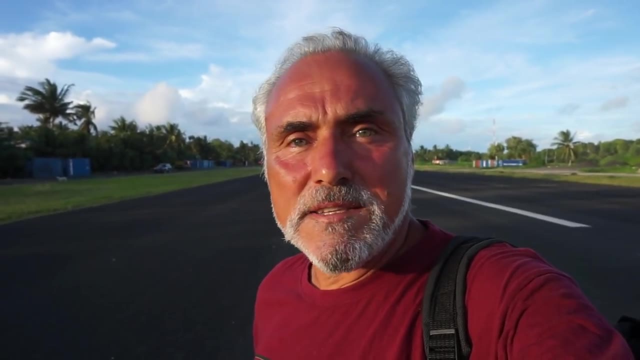 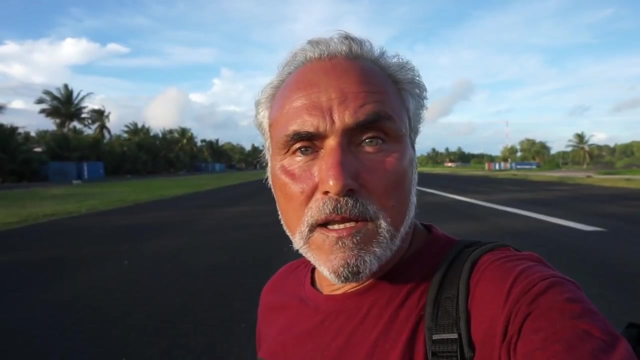 Now that was bound to create a lot of problems. Tuvalu or Ellis Islands were mostly Polynesian and the Gilbert Islands were mostly Micronesian people and they created a lot of problems. Eventually, in 1974, when the Queen of England was and she still is the Queen of England- was Elizabeth II in 1974, the two colonies split: The Gilbert Islands separated from Ellis Islands and now we had two separate colonies. Eventually both of them gained their independence from Great Britain. The Ellis Islands became independent on October 1st of 1978, and they were now recognized. 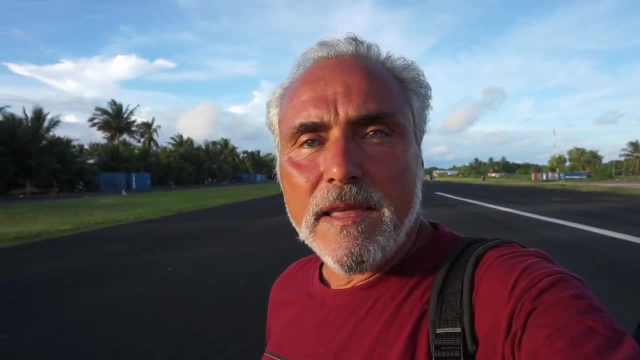 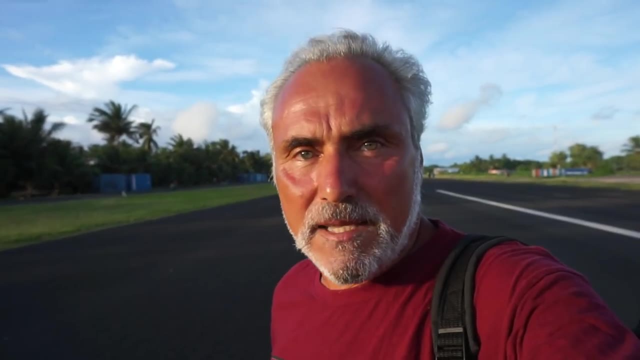 as the country of Tuvalu, where I am today. The Gilbert Islands became independent a year later- A year later in 1979, and now they are known as the Republic of Kiribati, And now they are two separate nations all together. 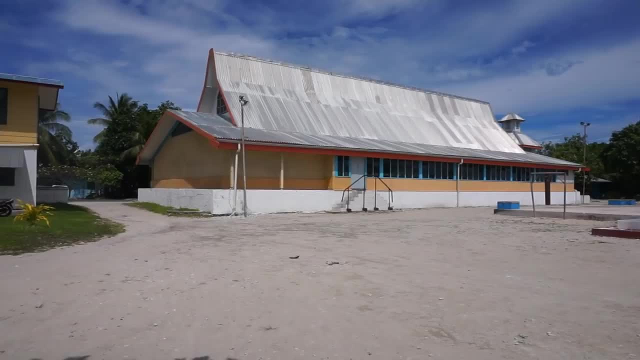 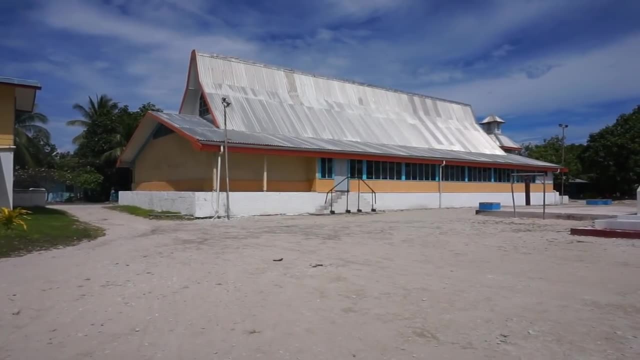 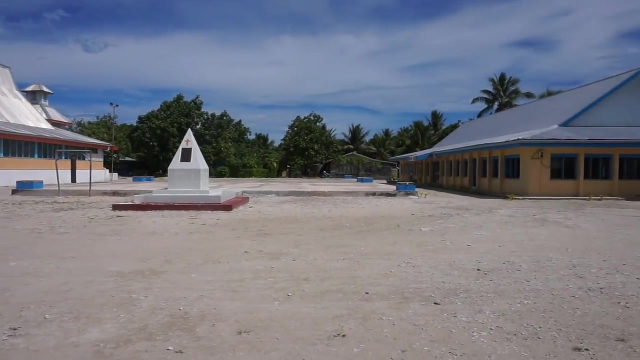 And here is one of the most prominent landmarks here in Funafuti, the capital of Tuvalu, And this is the Methodist Church, one of the biggest buildings, if not the biggest, On one side and on the other side, the community center. 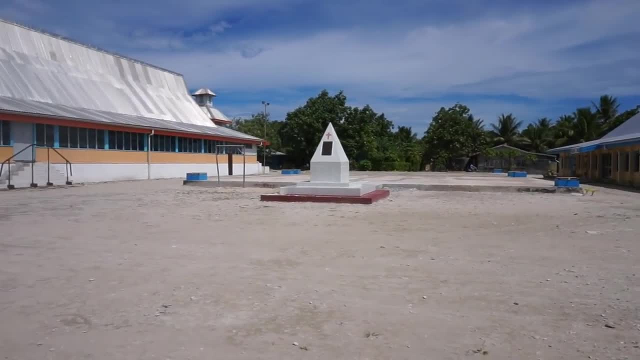 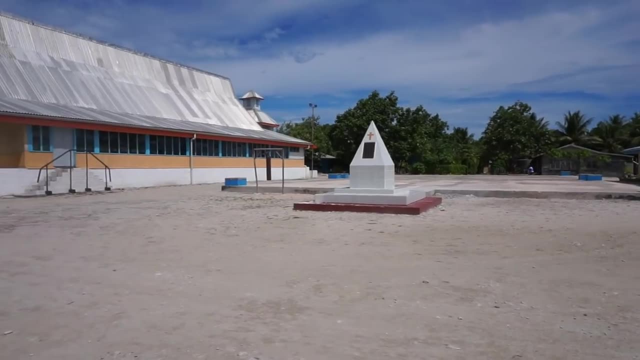 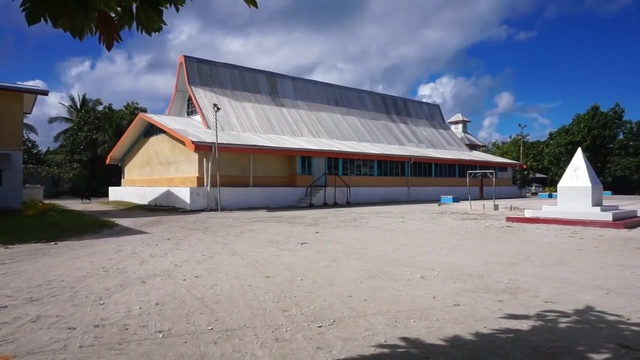 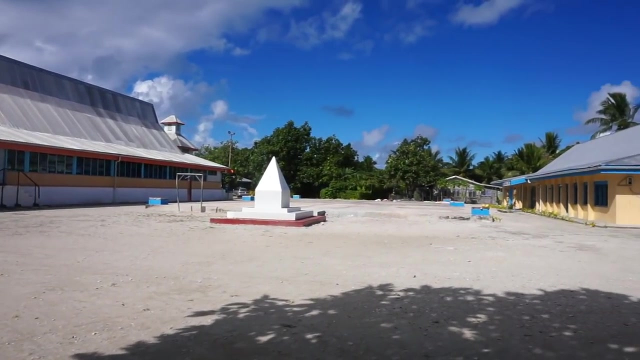 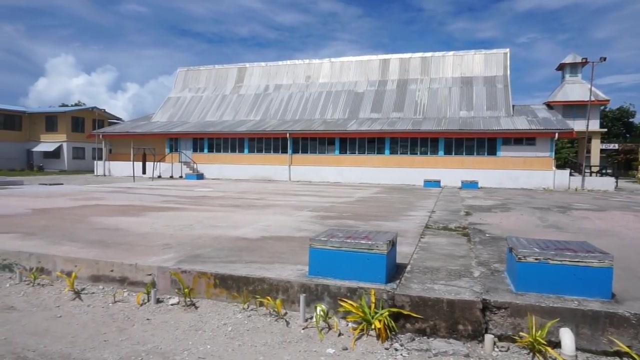 We're going to go on the community center. in a second Right, in between the two, there's a monument erected to the priests or pastors that served the Methodist Church since 1865.. And here's the Methodist Church. That's the memorial that we just saw. 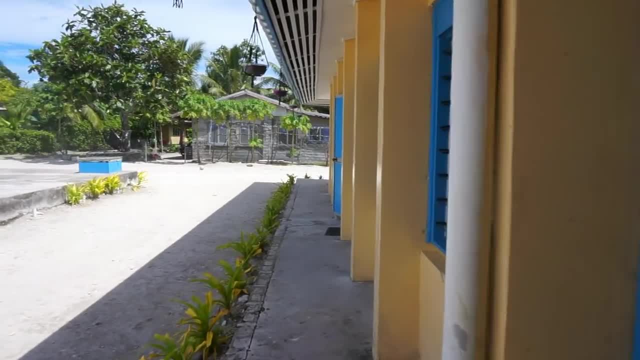 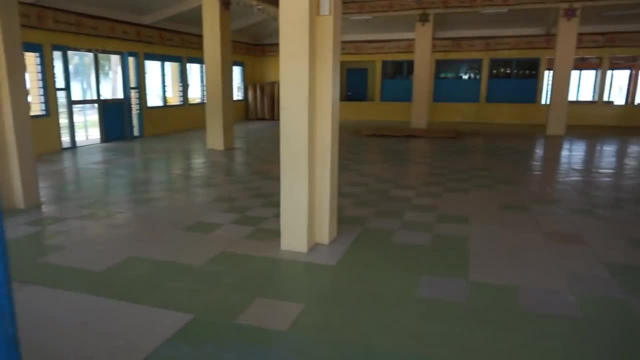 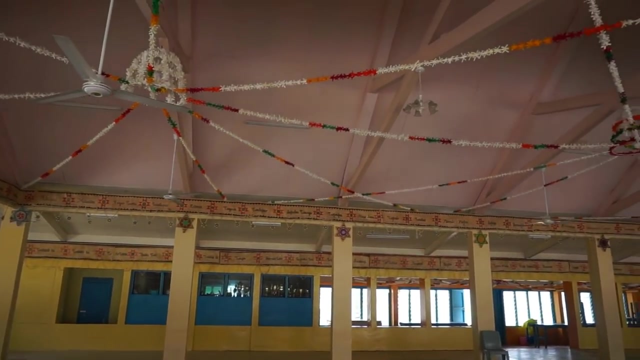 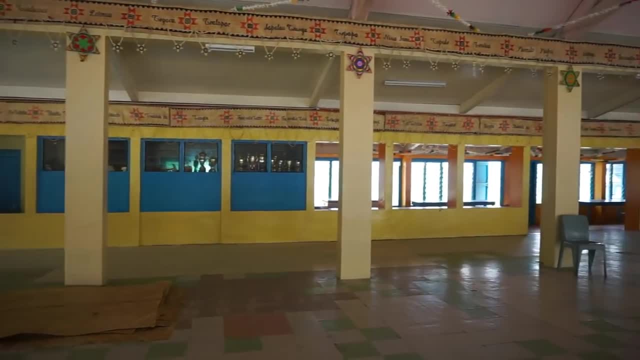 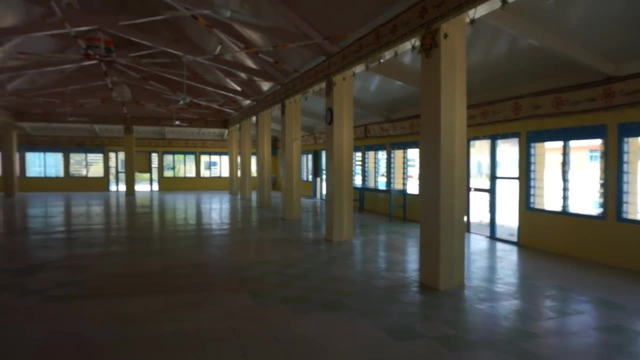 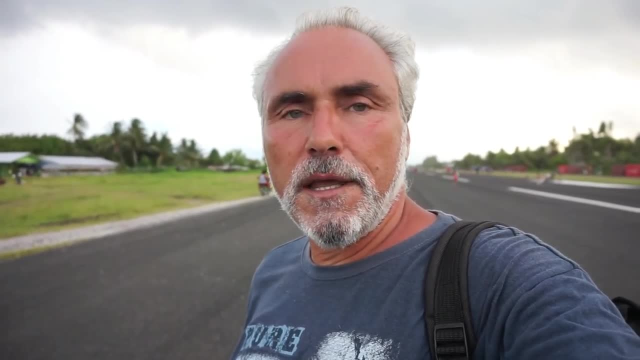 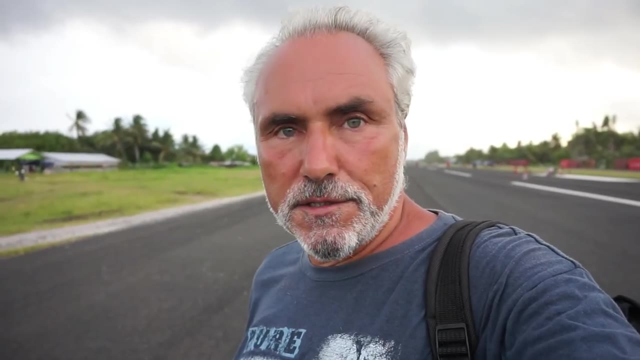 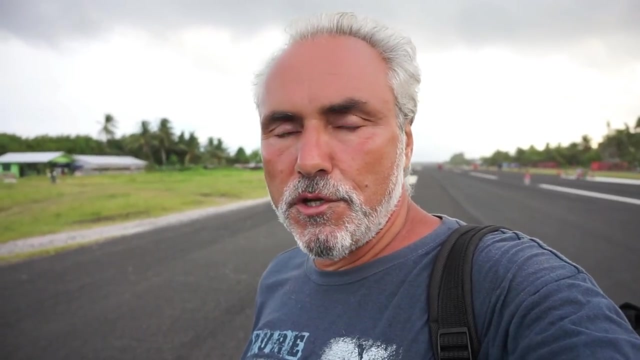 Another major source of revenue here for the Tuvalu people, Duvalian government, is the licensing of the domain extension tv. when the domain extensions were assigned to the countries a few years back- and let's say Australia got au and Italy it, Duvalo was very fortunate to get tv. 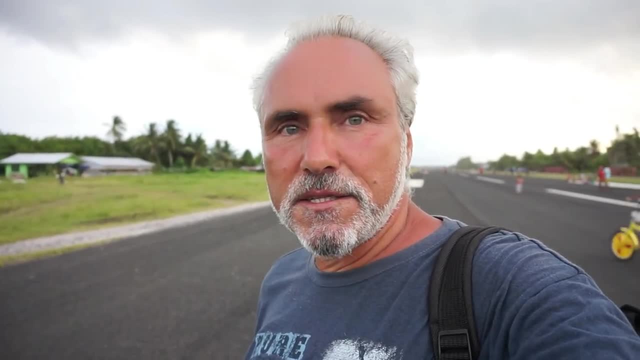 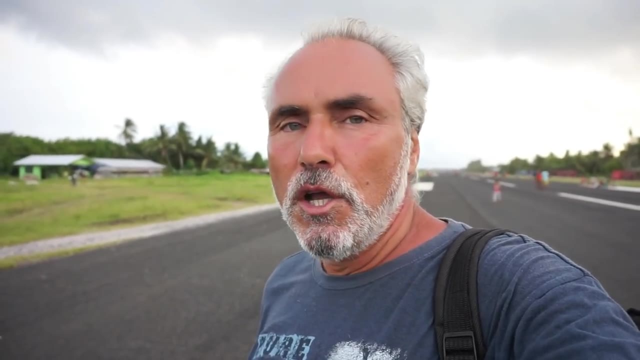 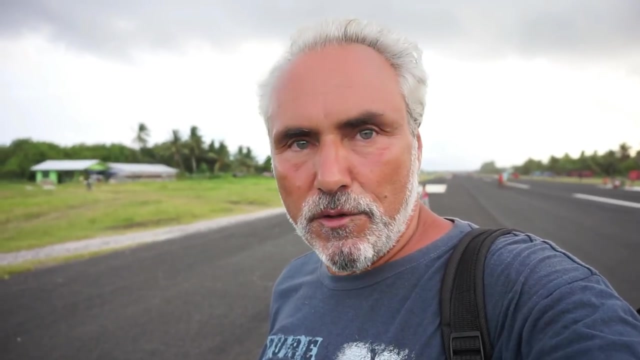 very quickly. they realized they could license that domain extension and they did so and, as a result, they have a major source of revenue by licensing the tv domain extension to companies like CNN. that's how you get CNNtv, for example, and that contributes greatly to the revenue on a year basis, because 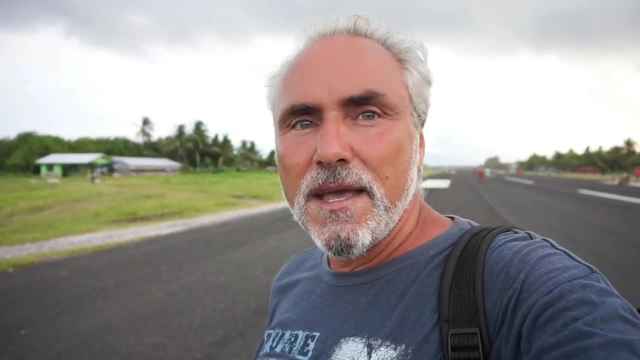 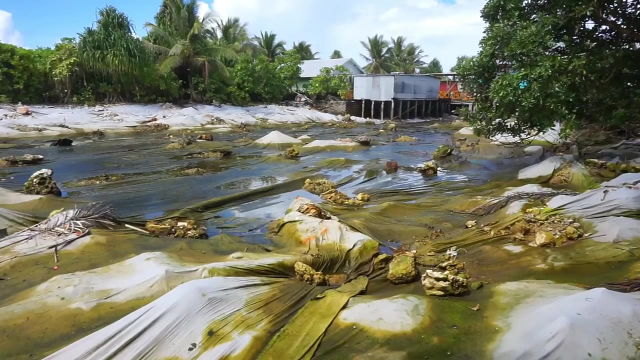 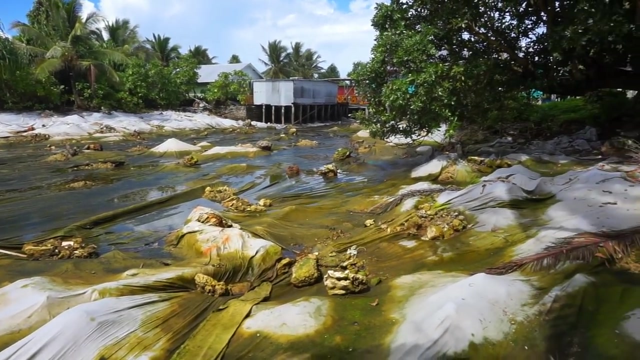 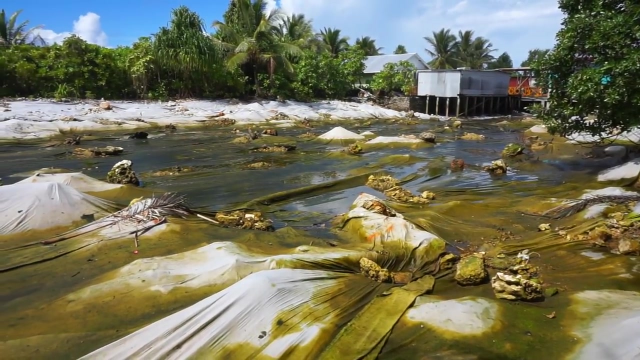 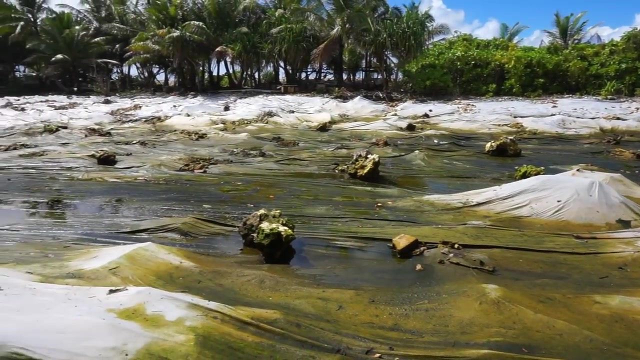 licensing the domain extension tv takes place on a multi-year contract and it helps the local economy here tremendously. and here is a very sad and very, very ugly side of Duvalo. you're looking at a pit which runs for a length of at least 300 meters. 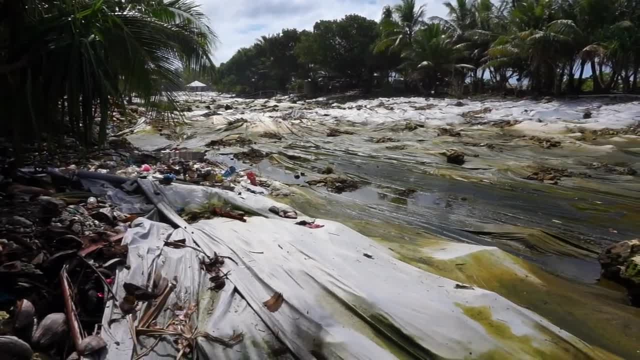 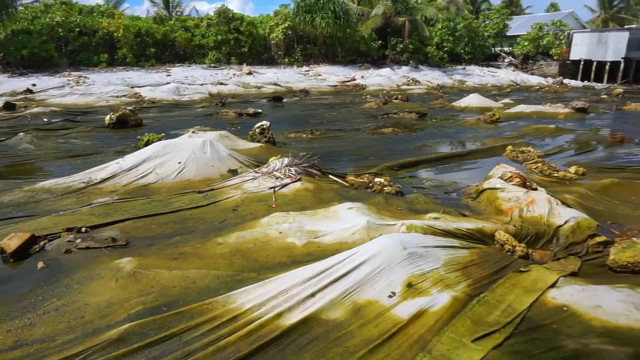 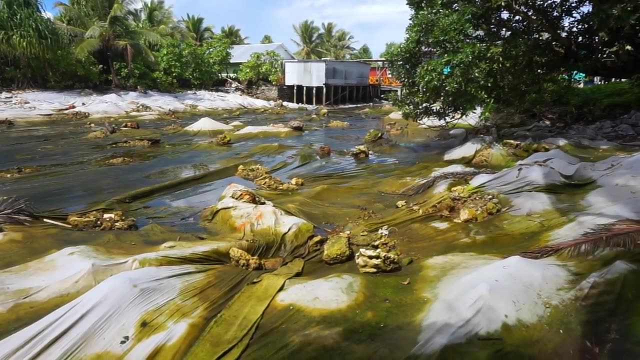 you can see in the far distance over there the extent of this pit. what happened here is 1942. the Americans moved about 6,000 Marines to Funafuti in preparation for their arrival in the United States. tv tv attack on the Japanese in the island of Besso, which happened in November of 1943. 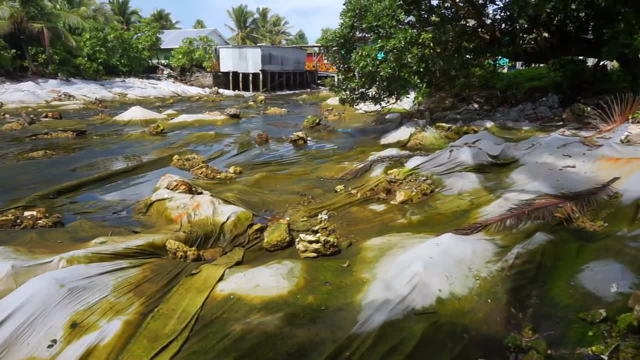 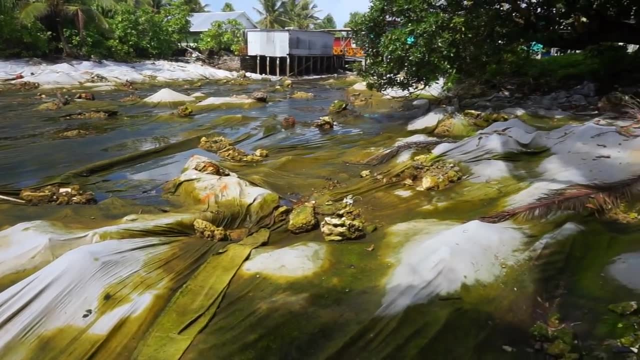 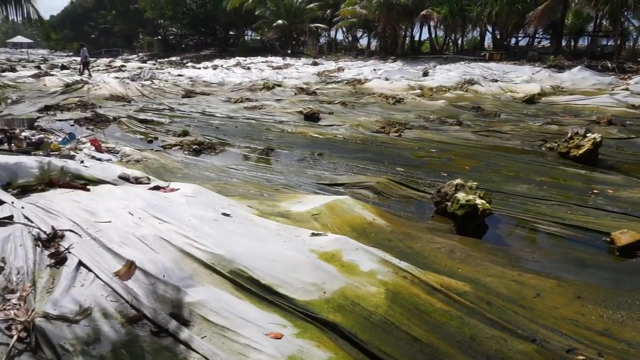 the attack that is against the Japanese and that is known today as the Battle of Tarawa t-a-r-a-w-a. well, that when the job. when the Americans arrived here in 1942, they dug up this huge pits in order to get rocks and sand for materials to. 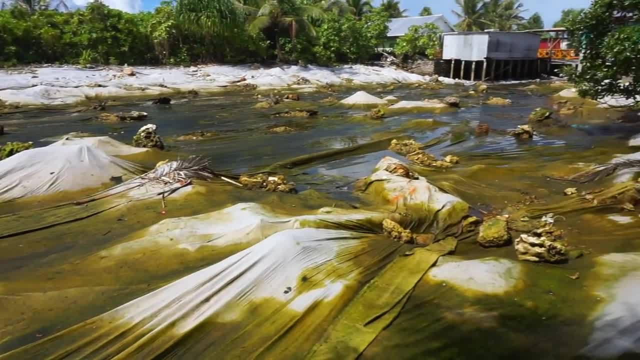 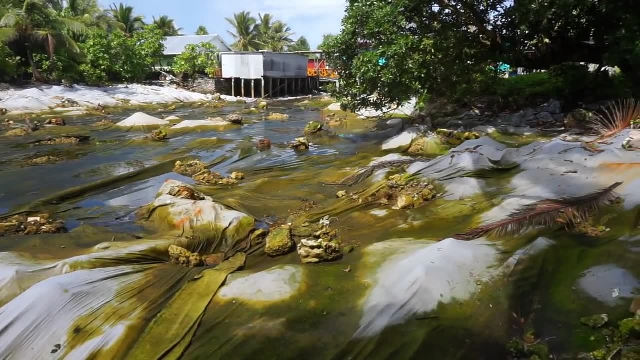 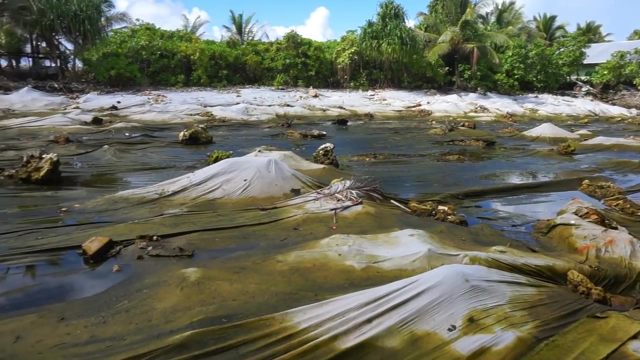 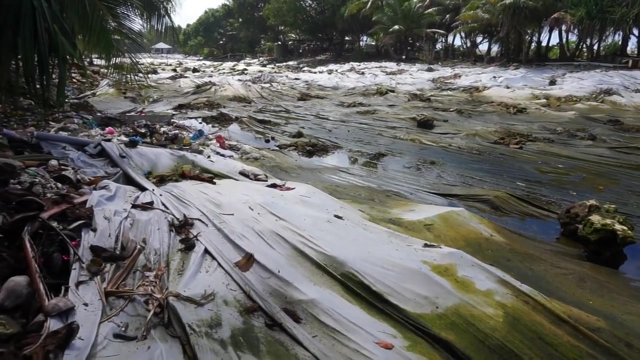 build the arch strip and other buildings that they needed and, as a result, over 70 years later, these huge scars on the eastern side of the Island. you can hear the waves right behind those trees. that's the eastern direction and his huge scars are left here. you can see the garbage over here. now, after the